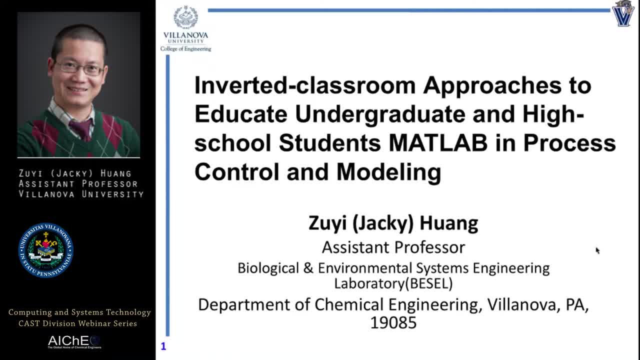 Yes, thanks, John, for the introduction and the invitation and to give this webinar. I'm glad to share the teaching modules I developed in the last two years and to educate high school and college undergraduate students and with the MATLAB skills in process control and modeling. 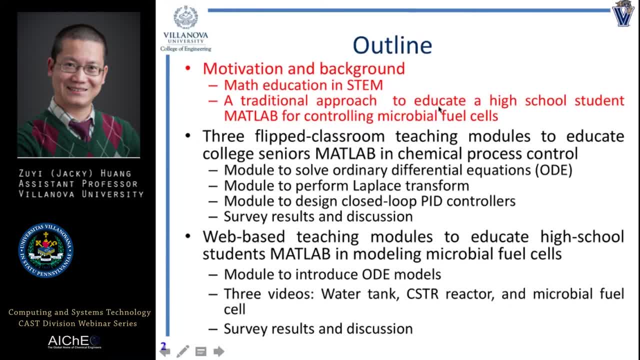 So here is the outline of my talk today. I mainly focus on three projects. First, I will introduce a project done by a high school student in the summer of 2014 in my lab, and that student developed optimal model for microbiofuel cell and he also played around with the PID controller design, and actually it's that project that's motivated him. 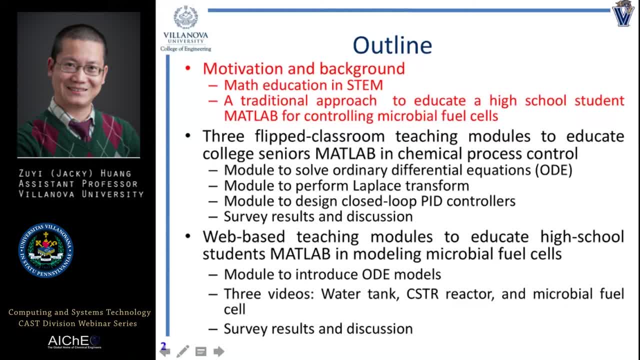 me to develop the flipped classroom teaching modules for the course I teach at Villanova, the chemical process control. So this is my second project. I'm going to show you today and I'm going to show you the modules, the three modules I developed in this course and also give you some feedback of the students in the 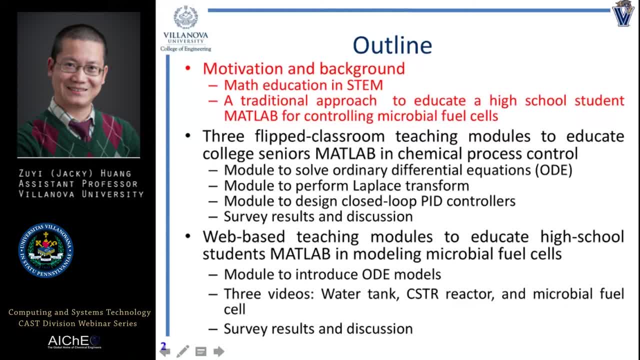 flipped classroom teaching approach And project three actually is an extension of project one. So in project one the high school students came to my lab and got training in person and did the lectures in my lab. In project three the students did not meet me and they watched the teaching modules from the internet and actually 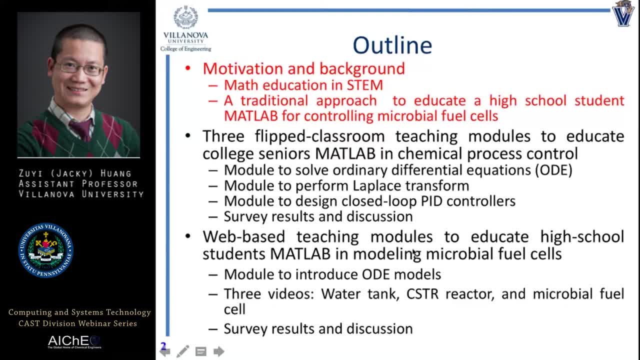 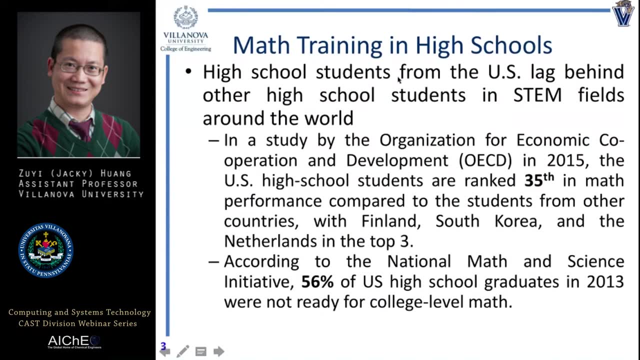 from YouTube and then we had a Skype meeting, So it's all web-based. I'll also show you some feedback from the students on this web-based teaching approach. Here is some background about the projects and to explain why I developed these teaching modules. So, as you may know, the mass performance of US high 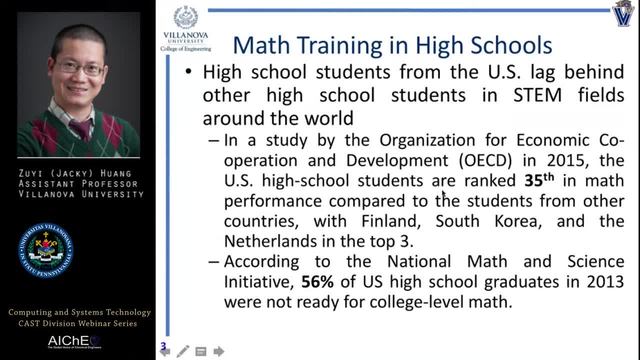 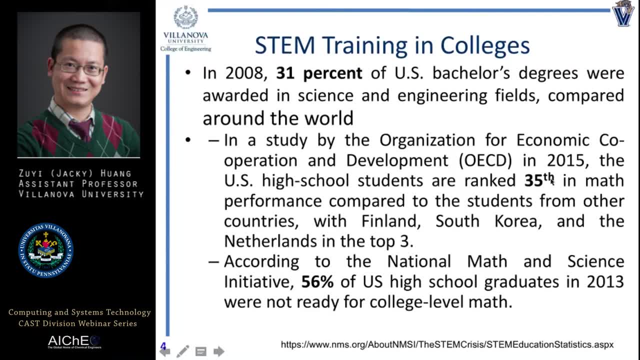 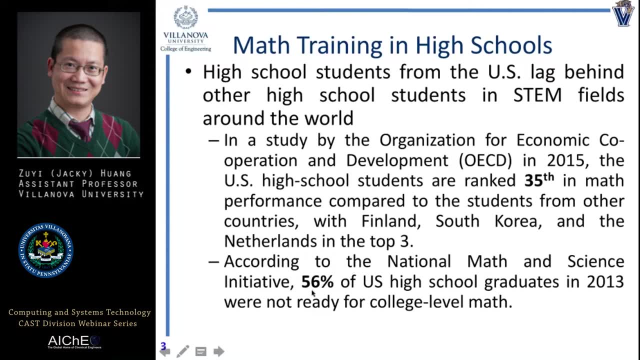 school students are not ranked top one anymore. Actually, they were ranked in the top 35 in 2015. And according to another survey here, 56 US high school graduates in 2013,. they were not ready for the college-level math, So you may wonder whether the situation 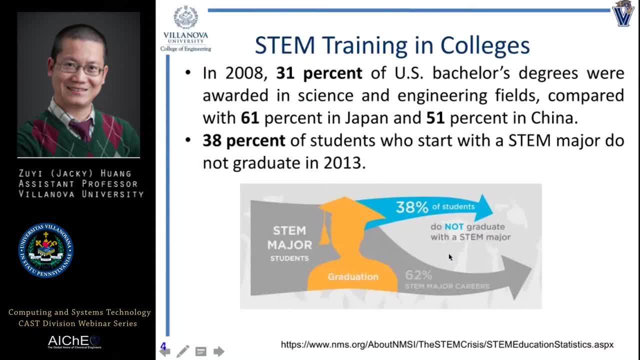 is better for college students. Actually, it's not better. So here is some information. compared to Japan and China In 2008,, we had much less students and were awarded in the STEM field. Even some students picked the STEM field as their major- 38 percent of them. 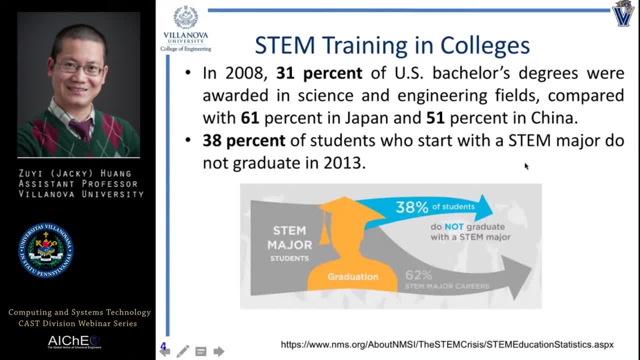 failed to graduate in time. So, as the teachers right in the STEM field actually in the process of control and modeling, I think we should figure out a way to attract more students to choose the STEM major. also try to make the STEM lectures more fun and more cool to students. And so one idea come. 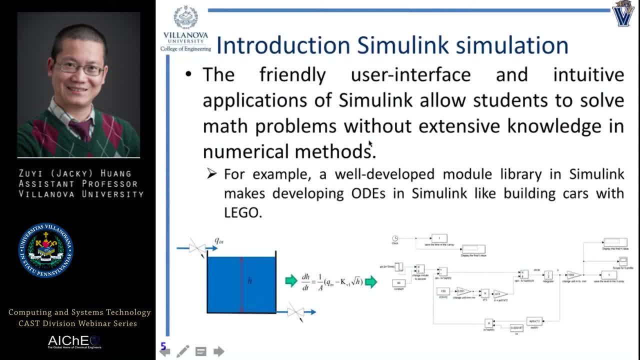 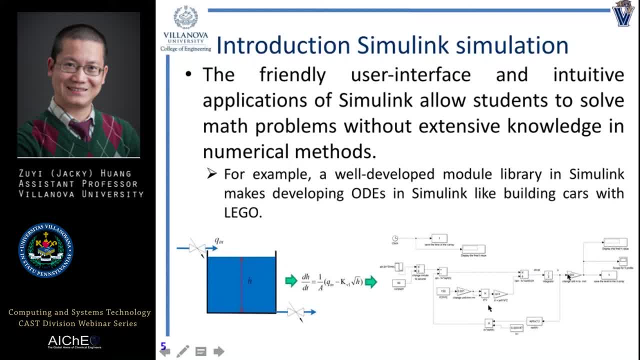 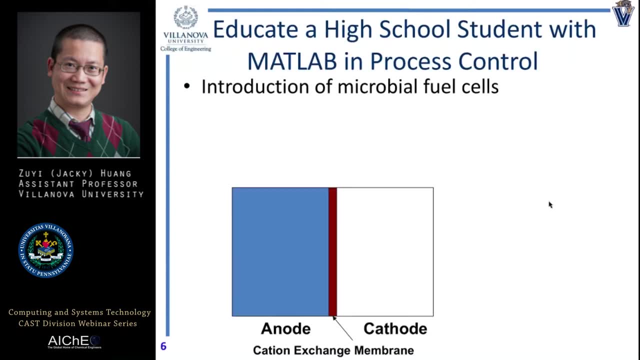 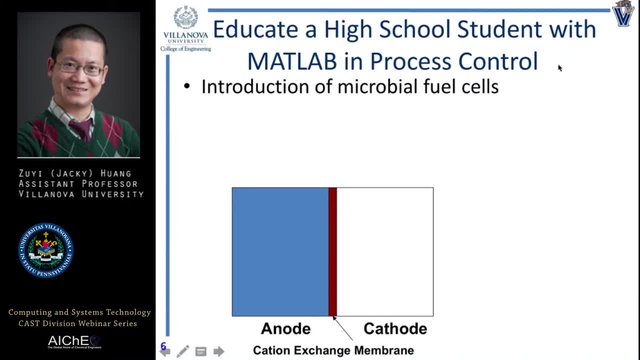 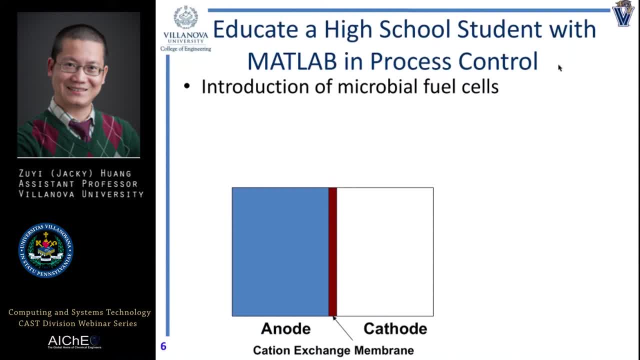 Thank you. I would like you all to know why driver accident occurred in my city. Thank you, �EN𝛰𝄞𝕥𝕝𝕞. now I would like to offer another educational perspective and drawing tepid speech. 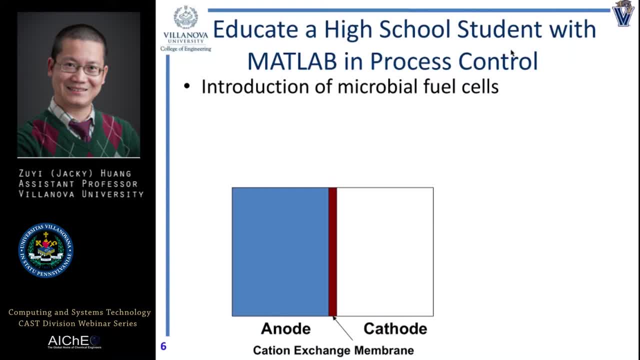 for the guests Thank you project to the students right in the summer of 2014 and the student was more interested in microbial fuel cell. and now I want to show you a brief introduction of microbial fuel cell if you are not familiar with microbial fuel cell. 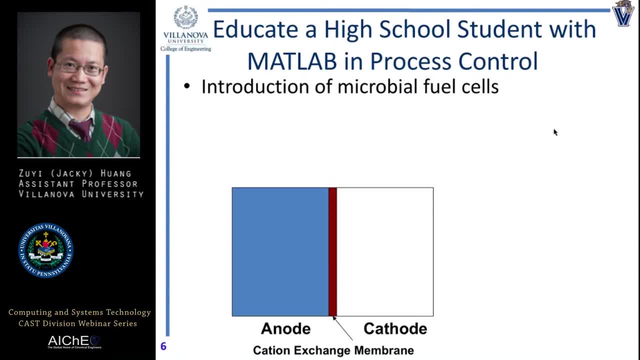 So similar to traditional bacteria. we have anode and cathode, but, differently, we grow bacteria on the surface of the anode and these bacteria are specific bacteria that are actually called exoelectrogenic bacteria and can produce electrons from organic compounds, from wastewater. 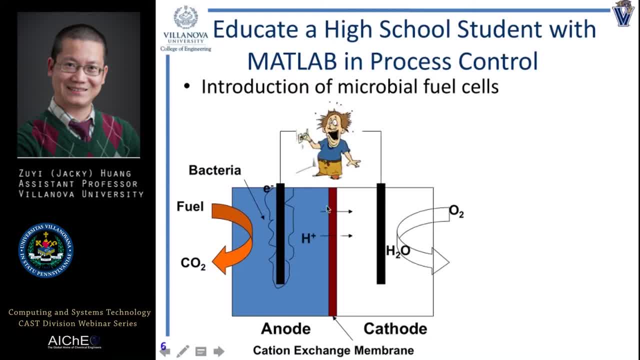 and this is a little cartoon to show you the mechanism of microbial fuel cell and you can see that organic compounds are converted to carbon dioxide and electrons and protons, and then electrons translocate through the external electrical circuits to the cathode and then react with protons and hydrogen to produce water and these are electrons in the anode. 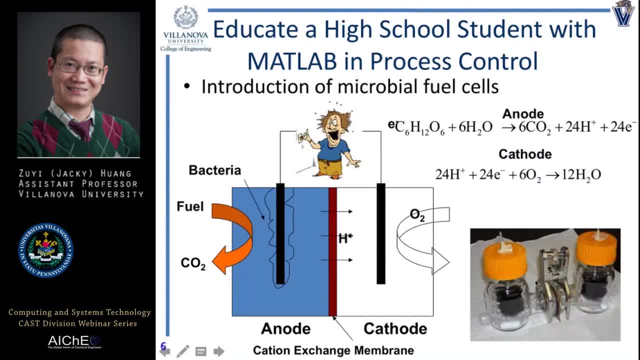 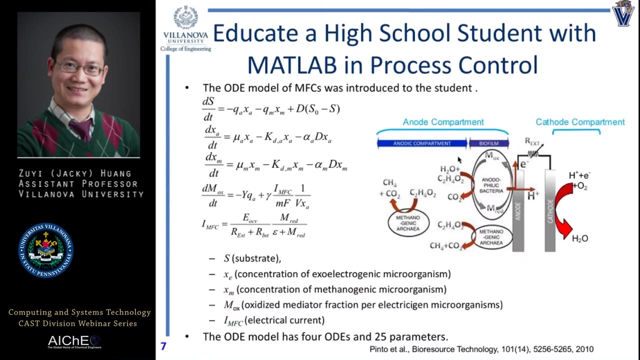 and cathode and this is the water. So this is what the microbial fuel cell looks like and you can see that microbial fuel cell provides a sustainable approach to treat wastewater and, at the same time, produce bioenergy. and the student, he was very interested in this project and then after that, and then I introduced 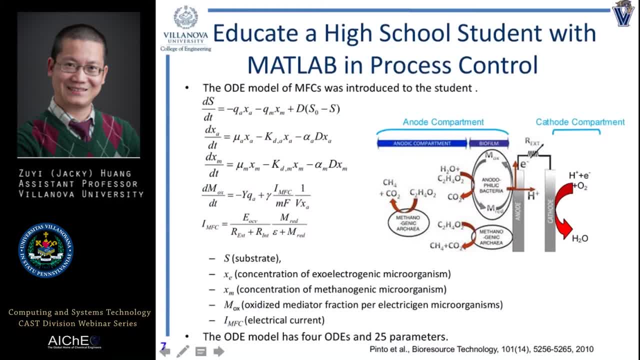 the OD model of the microbial fuel cell to a student. Well, due to the space constraint I don't show you the whole equation and of the model, and here just a brief introduction of the model. So this OD model describes the concentration of the substrate in the reactor and also the 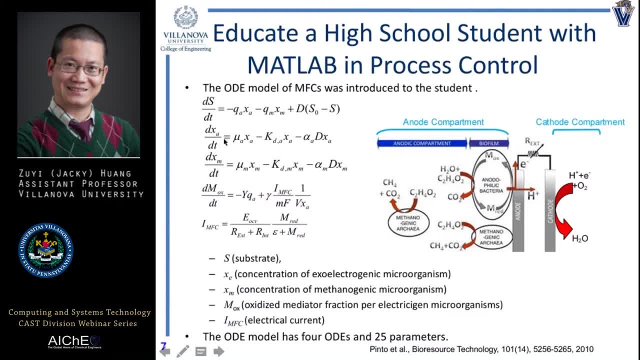 population of the exoelectrogenic bacteria, by which can produce electrons from wastewater, and another one another bacteria- here is a methanogenic bacteria. So this is the first one, This is the second one, This is the third one, This is the fourth one. 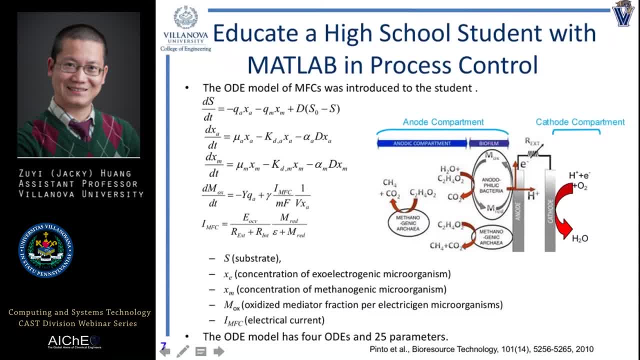 This is the fifth one, This is the sixth one, And they can produce electrons. And also we had the equation to describe the proteins inside the cells that carry the electrons from the cell to the anode surface. right, because of the data. 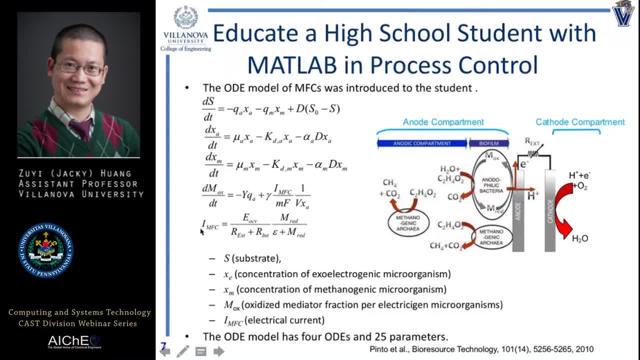 And also we had the equation to quantify the electrical current signal. Now, actually, some coefficients. for example, this goes away in mu A and goes away in mu M. They are the function of the substrate. We have nine more equations for all these coefficients, right, and I don't show them. 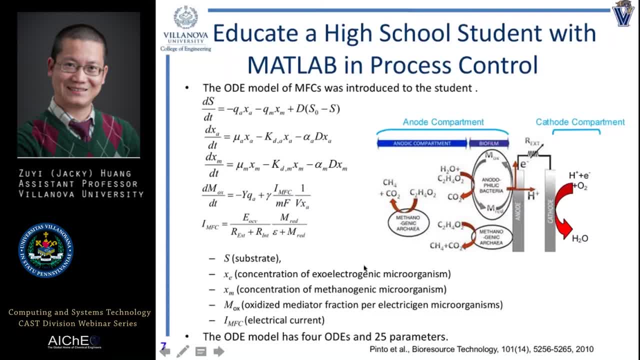 here. But anyway, this model is pretty complicated and it has 25 parameters So I want to test the student. all right, if the student can. high school student can handle this complicated model All right And in some link. so this means that it's doable to introduce the link to the high school. 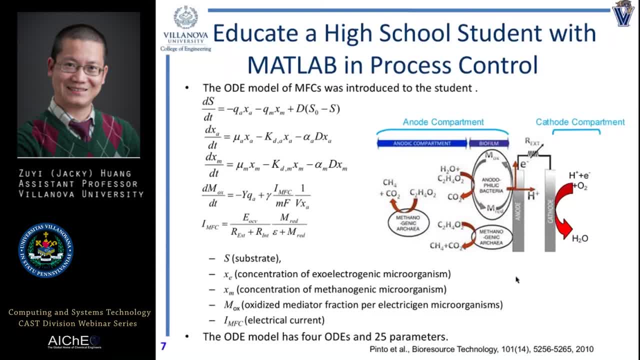 student and then to right to let them to do some research and then maybe work. And then I charge more students to stay in the same field, especially in modeling field. And well, when I introduce the ODE model, I will explain the physical meaning of each. 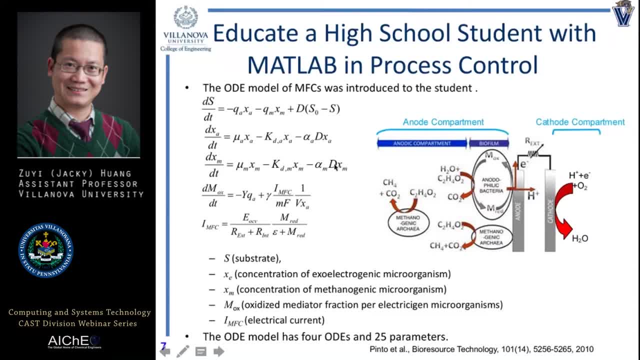 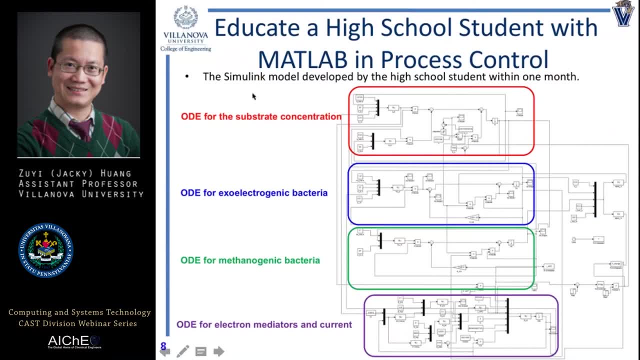 term. So you must understand what is the ODE model? I'm just going to do an example. So I started at the hospital. I was just one of the mid-20s. We were still in the school. I presented the ODE model to the students and understood the model. 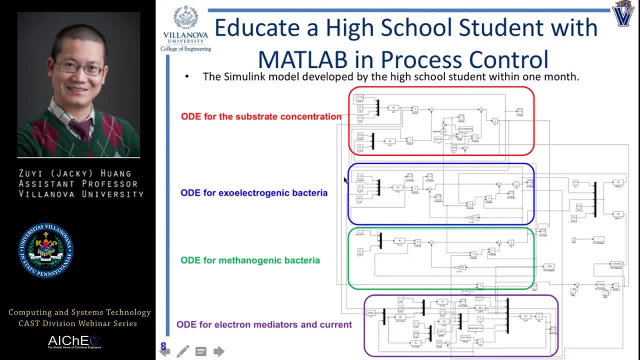 So after that the student walked two days in one week and in my lab and we developed the ODE model for right for different components right, for example, right substrate concentration and different bacterias and also the mititis and cholestinol. 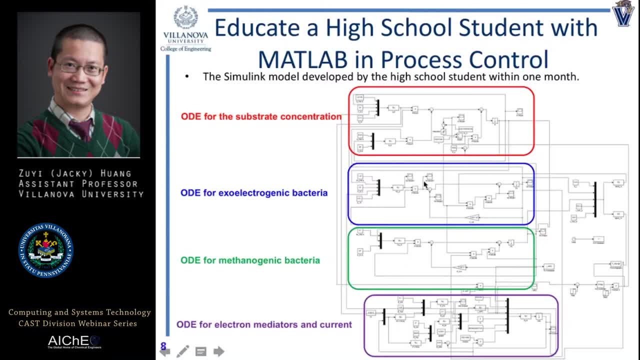 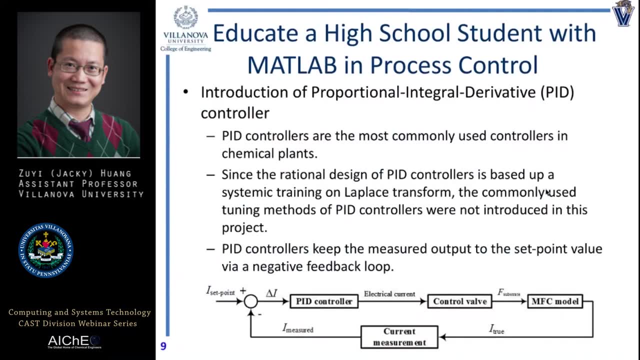 And then they spend one month And he got the model done, his model and using my model and verifying that his model is correct, right And well. so the student, actually his performance is much better than I expected. so I then wanted to further challenge the student. 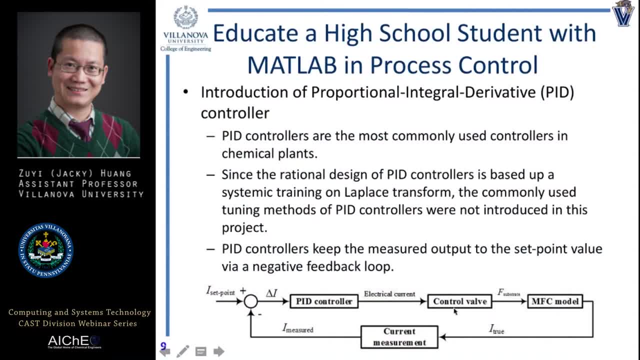 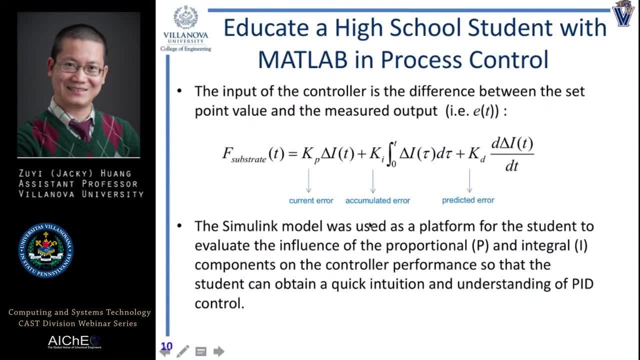 So I introduced the feedback loop right- negative feedback loop to the student and also the PID controller. Well, as you know, it's too challenging to introduce Laplace transform right to the high school student, So I did not do that right. 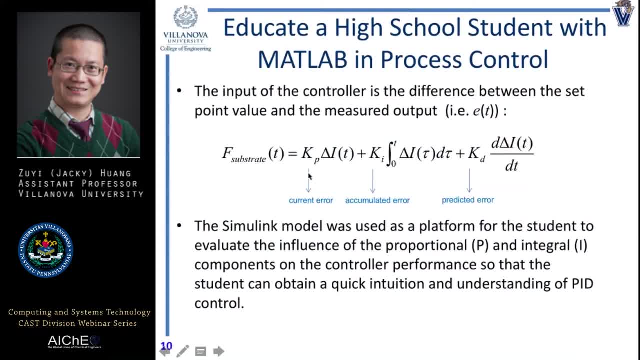 But I introduced the physical meaning of each turn in the PID controller And then I showed the student how to build a PID controller in Simulink and then the student can play around with the KP and KI and KD so that he understood the PID controller. 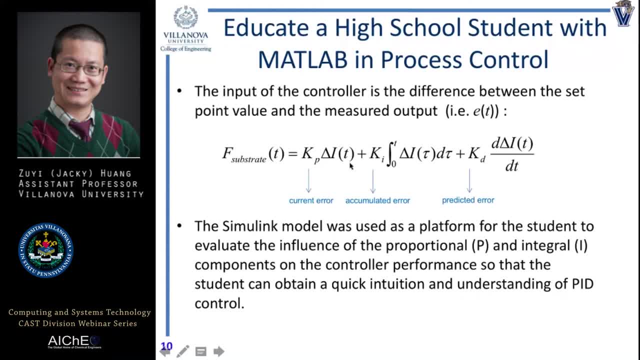 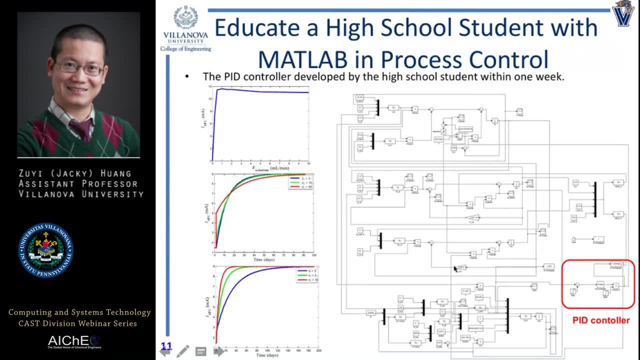 and how PID works and how each turn affects the PID controller's performance, right? So anyway, he spent another week and then he built a PID controller and then, right here are some results from his project. and he got the simulation results for different KC values. 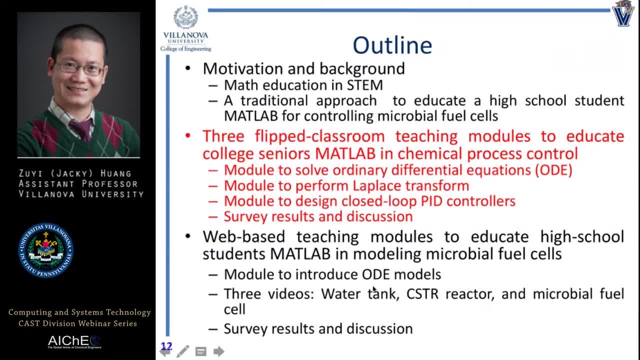 and KI values And the project. Okay, It's pretty successful, and the student actually. he gave a presentation in the ASIC Mid-Atlantic Conference in 2015 and so his presentation is very good, And also he got an offer from Cornell University, but he ended with the University of Pittsburgh. 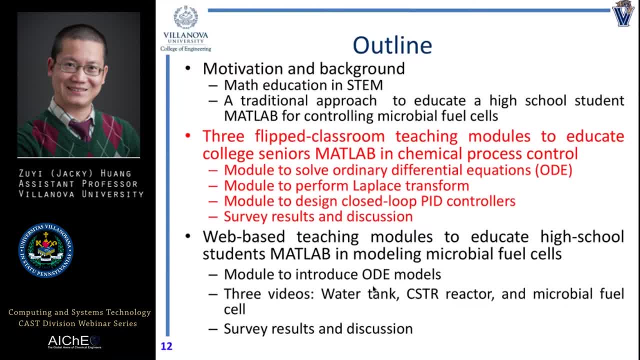 because you picked and offered him scholarship. Anyway, he's very good. Anyway, he picked the STEM major, He picked the Bioengineering major. I'm very happy with that. So now I want to move to the second project and then I want to show you before that I 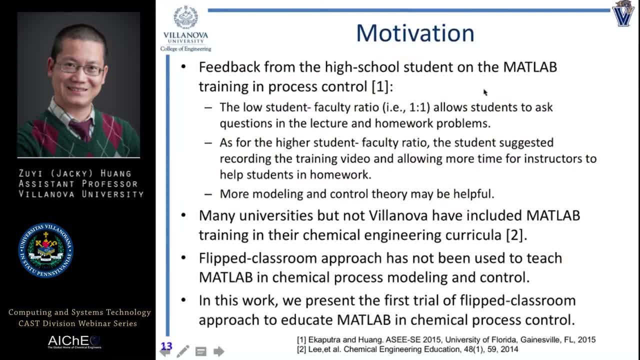 want to show you how I linked the first project to the second project. So, as I mentioned, the student, a high school student, did a great job in the summer of 2014 and I talked with him in person and then he gave me some feedback. One thing I want to point out is that in the summer of 2014,, I talked with him in person and then he gave me some feedback. One thing I want to point out is that in the summer of 2014,, I talked with him in person. 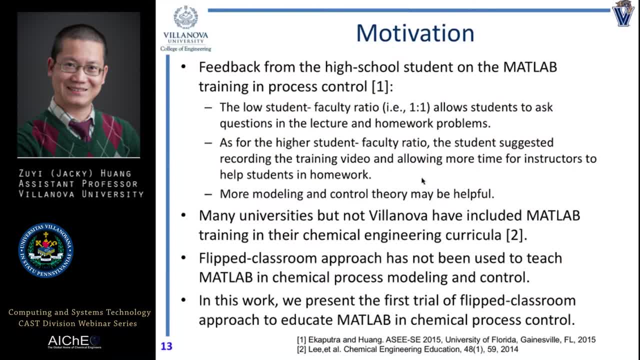 And I talked with him in person And then he gave me some feedback for the first project. What he gave me is that maybe I should call the teaching modules right and then more students, more high school students, can watch and then to run the link. 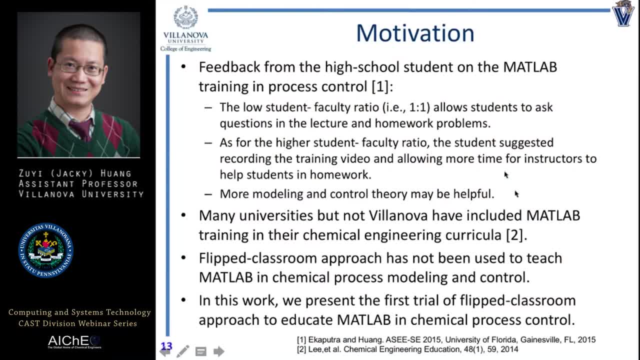 So that's why I did that. So that's why I did that. This is one reason. Another reason is, as you may know, Whatanoa is known for teaching And the faculty at Whatanoa are taking the courses They want to learn. 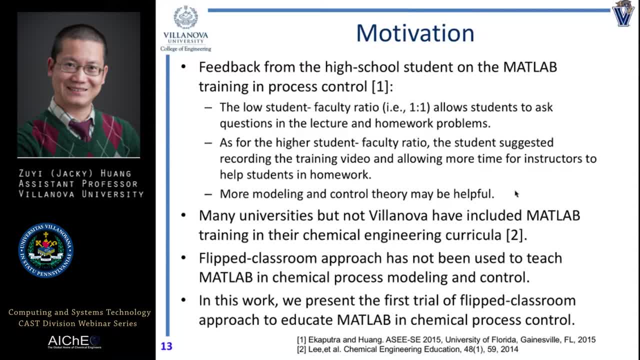 They want to do. they want to do, they want to learn. So this is the first project- has a great passion to use innovative teaching approach in classroom. So in the last few years we have some faculty testing the flipped classroom teaching modules. 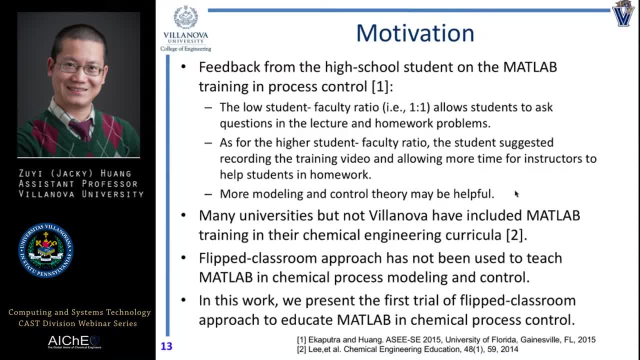 in the courses at Villanova, And so I have some good colleagues who did the experiment with the flipped classroom teaching approach. That's why I also hey, maybe I could try the flipped classroom teaching approach in my class by person control. So this is the motivation. 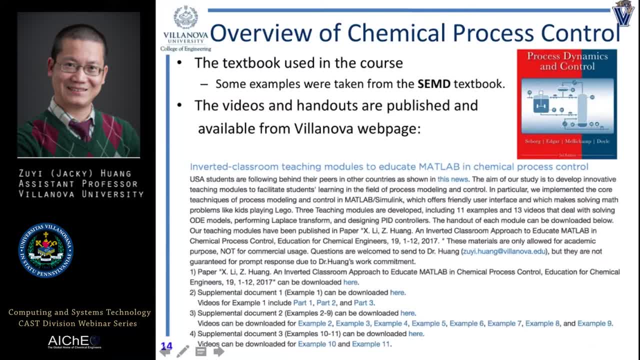 So now I want to show you the textbook I used. So I used this SAMS textbook right by Dr Seberg and Egger and Millichand and Doyle. Well, for me, the test book actually was a good book. 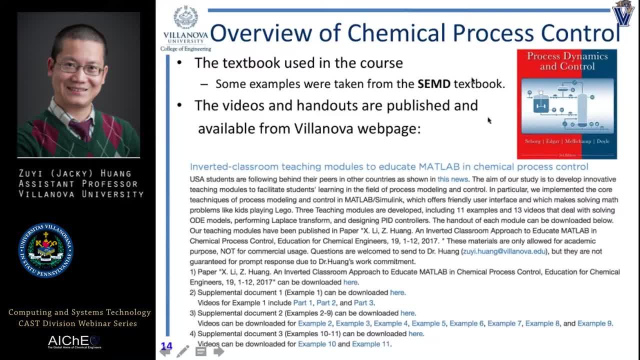 And actually my, My PhD supervisor is Dr Jorgen Hahn. Actually, he is the PhD student of Dr Egger, So that's why I used this textbook, because we have kind of an academic tree here. Anyway, the students also like this textbook. 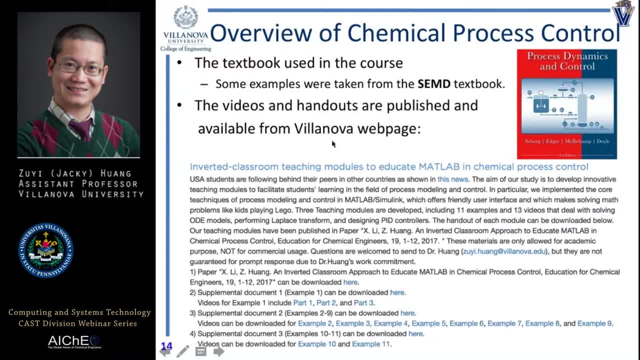 Again, as John mentioned, we already published the teaching module in a journal here. So this is the journal And actually in In this year, And so if you want to get the handout, you also can get it from the website of Villanova. 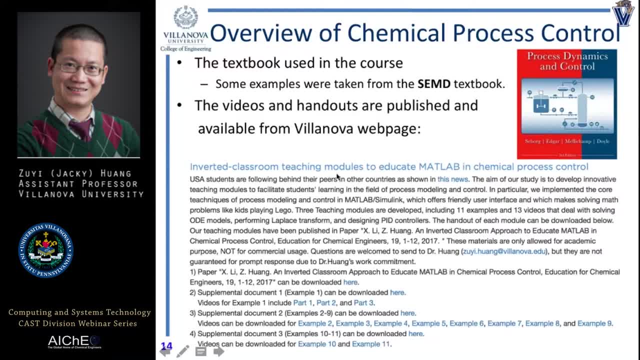 You could just Google my name and then go to my group website and then you go to the education category And then you could find either supplemental document for different For three modules, for each one, And then I also posted the videos So you can go to the YouTube. 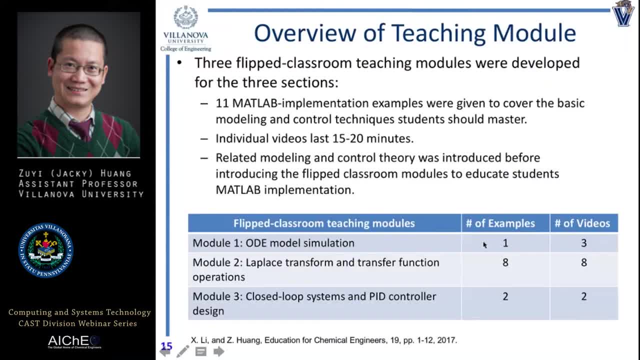 Yeah, Okay. So here is an overview of the teaching modules, And so we have 11 examples and three modules. So the first one is about solving ODE in instrument link, And actually I show students how to solve the CSTR model. 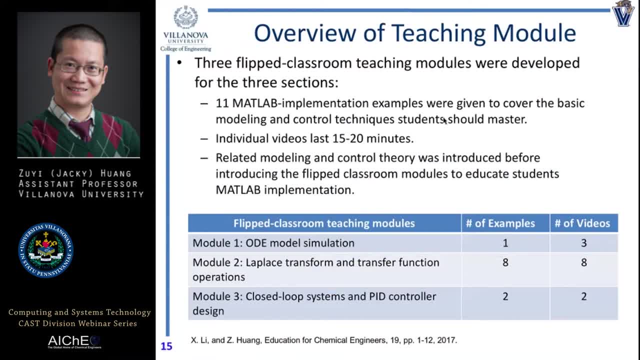 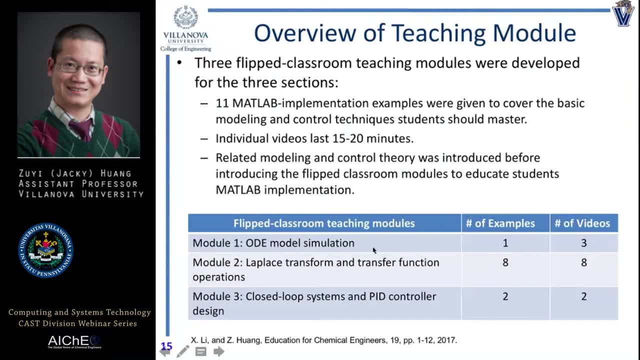 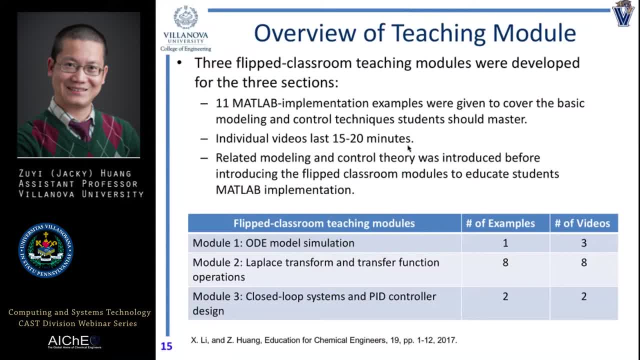 Example. So again here, the individual video typically lasts 15 to 20 minutes, And the reason for this is my colleagues at Villanova. they do a lot of experiment on the flipped castt jeans twin approaches, And the data shows that the time between 15 and 20 minutes is the best. 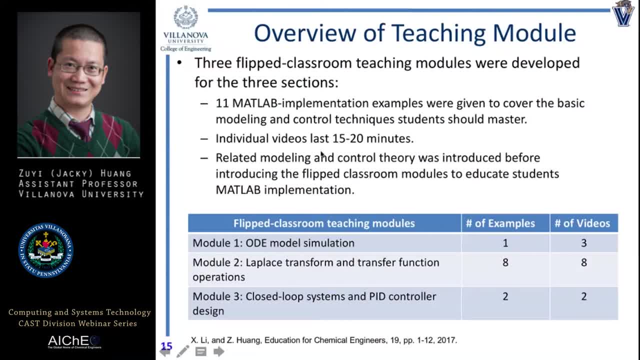 Okay, I try to make the videos for this time duration, And so the second module is the LAPATRA form and transfer function operation, and we have eight examples And then for each example we have one video, and the last one is more about closed-loop. 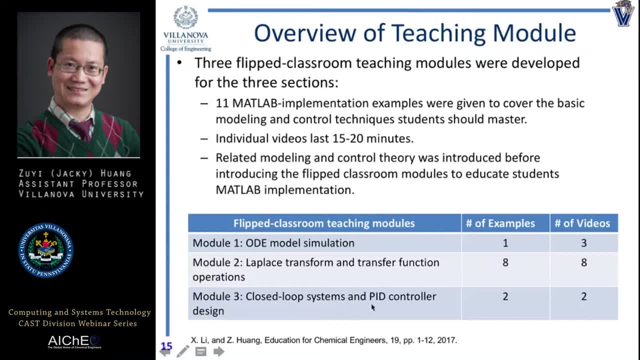 systems and also periodic control design. so we have two examples and two videos. So before I introduce these teaching modules to a student, I did finish the introduction of the modeling and control theory, so the student only knows the control and modeling theory before they learn how to use math to solve the problem. 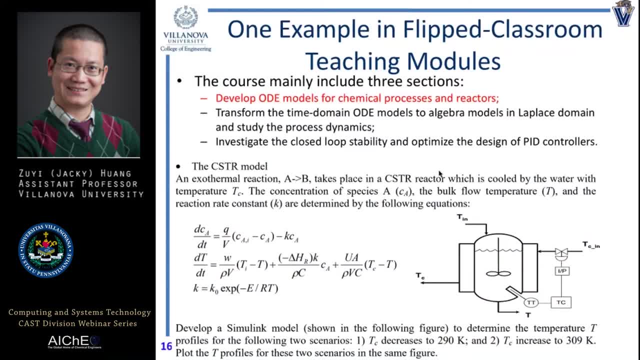 So now I want to show you more detail about each teaching module. First I want to show you how to write the module to solve ODE in Simulink. So here is the CSTR model I introduced in the class, So I will – so, for example, for the concentration ODE right. and then I show students how to 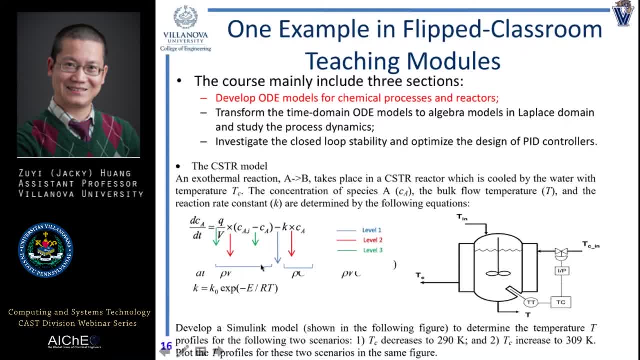 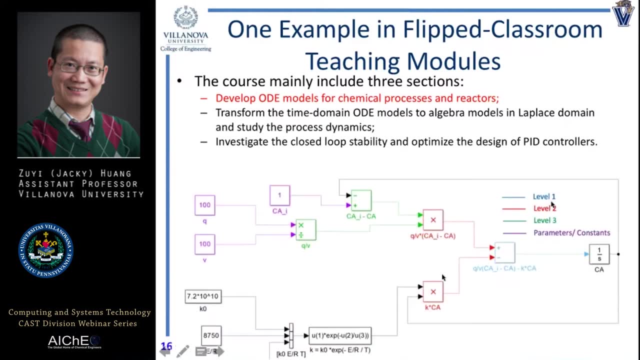 break the ODE into different right, different levels. right, for example, level one is the minus sign and then after that, level two. here is the product right and this product and then another one, so that we could – so that we could represent the ODE right in. 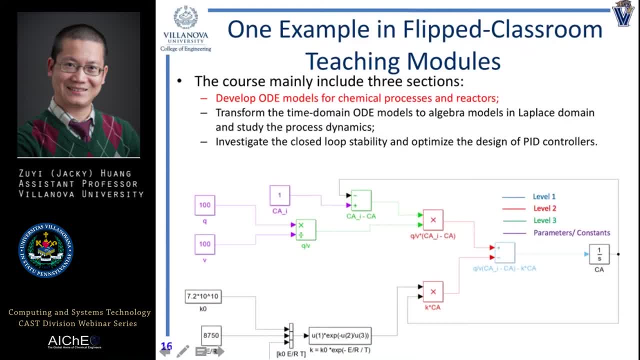 different levels, right, and actually just like how can we break the ODE into different modules and then we could use those modules that are available from Simulink and to build the model. So I show the students step-by-step in the video how to do that. and then – and most 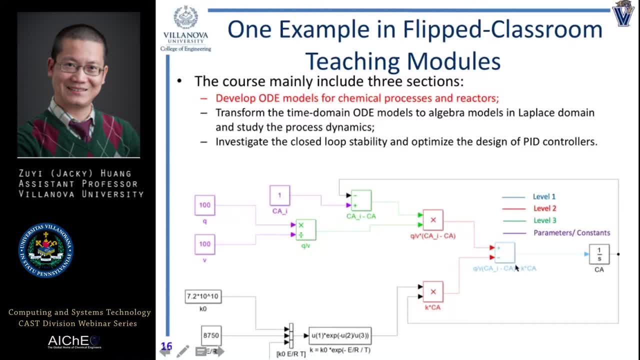 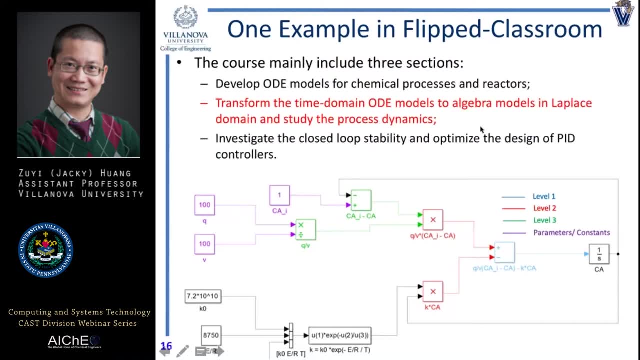 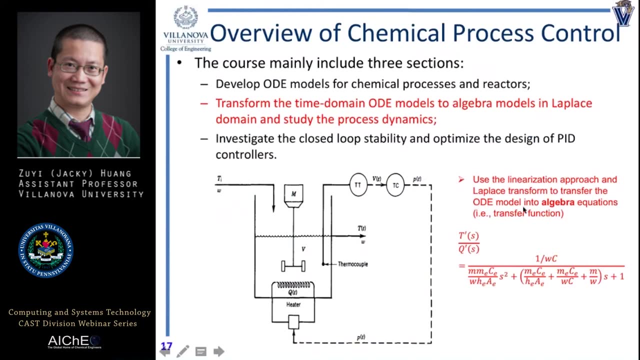 students can reproduce the result and just by watching the video. So this is module one. Now I talk about the module two and right. so in module two we try to – we try to translate the ODE model right in the time domain into the Laplace domain and which. 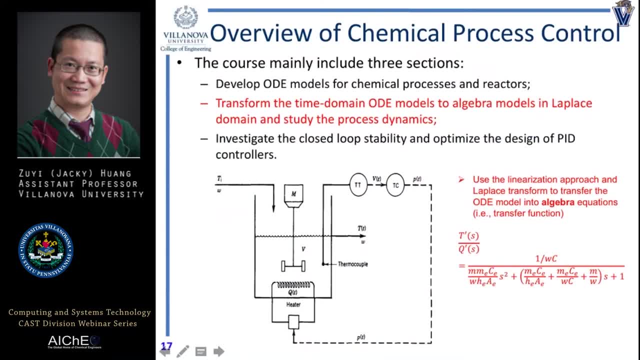 we're going to get algebra equation look like this: And well, it's very challenging for students to do Laplace transform or also to solve inverse Laplace transform right, and I will show you example later on this. And so, after we get the trans function and we also show how – what the output look. 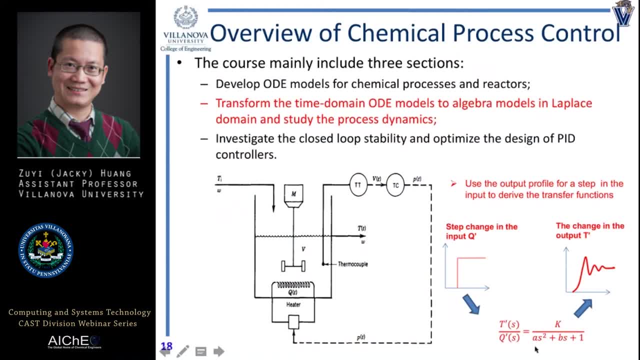 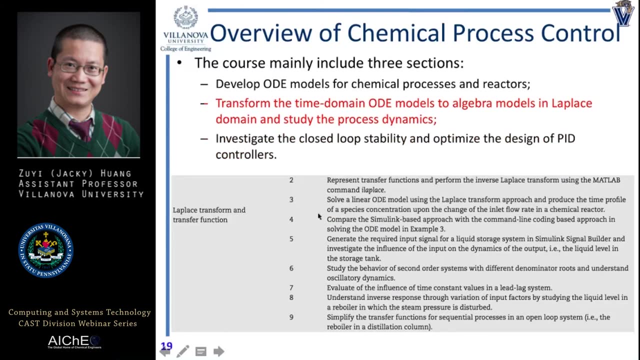 like for different inputs right, and also the A- B value right. the denominator of the trans function also will influence the system's behavior, And so this are the example I show and for the Laplace transform and trans function. So I want to show you a little bit more about the handout here. 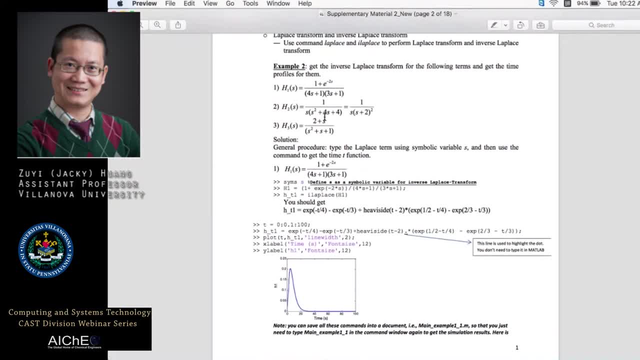 So, in example here – Yeah, I just had one question for you. Okay, Just as you're – you know, as you teach these students how – do they have prior MATLAB experience before their – this course, or is this the first time you're teaching? 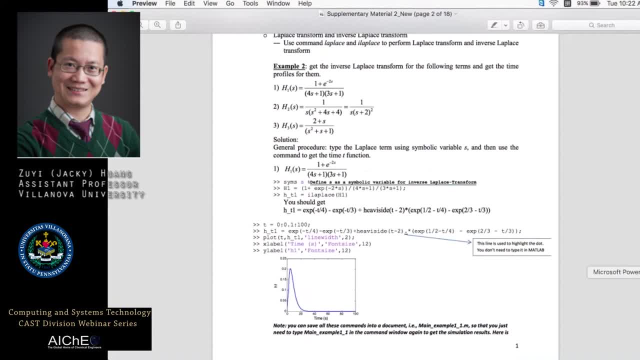 them MATLAB? Very good question Actually. yeah, very – I should mention that in my – you know my motivation Actually, the student at Vancouver and especially in chemical engineering, and they learn very little MATLAB Okay And in – right, in first three years it is kind of they don't know MATLAB that much. 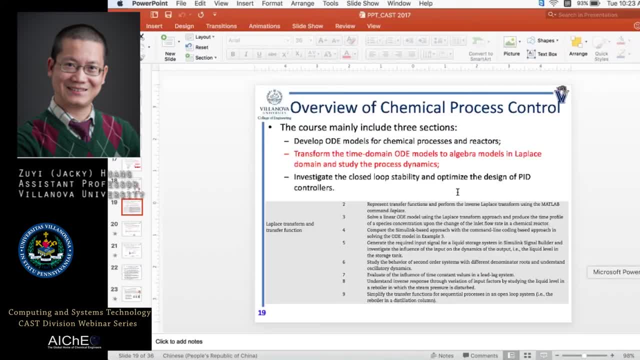 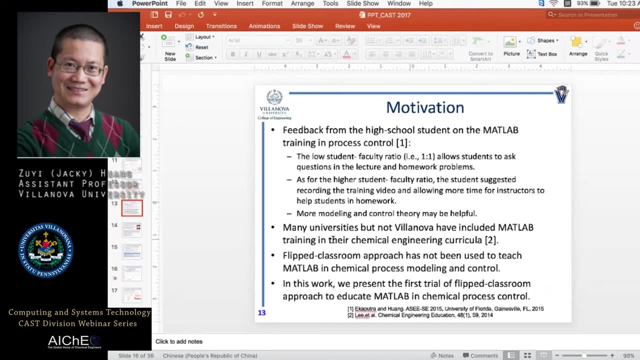 when they learn my course. Yeah, I forgot to mention this Actually. yeah, let me show you. I have one slide on this. I forgot to mention, and actually we see here, many university actually – but not many of them have include the MATLAB in their curricula. 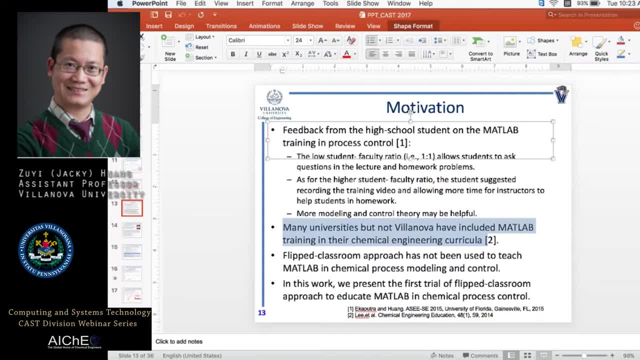 And we don't know how to do that. Okay, And we did a survey – yeah, we did a survey in 2014 on this, and that's why I talk with the department head- say, hey, we should right, include the MATLAB right and provide. 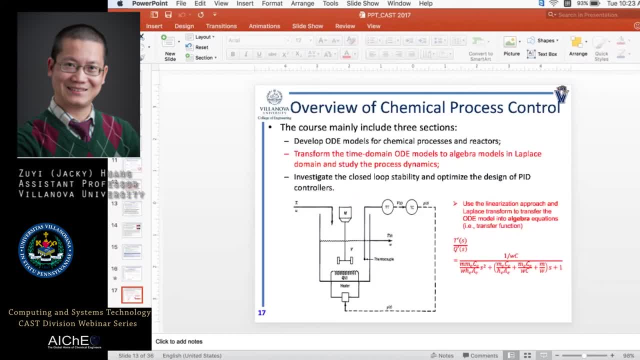 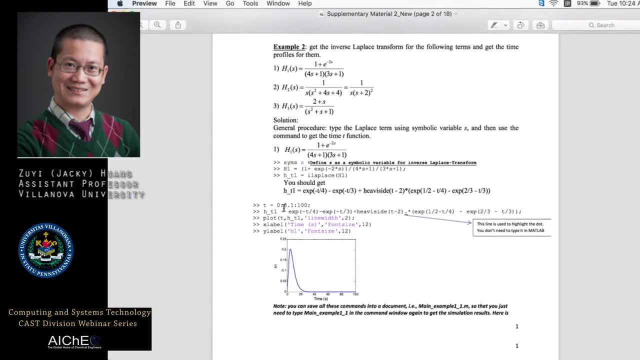 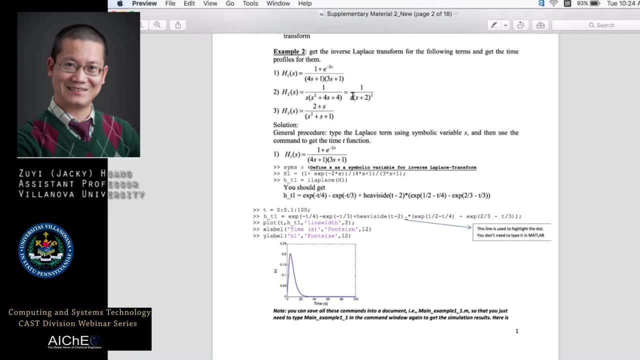 more MATLAB training to students. Great, Yeah, Okay, Yeah, Good So – see here So the – so example two – like example one is more about ODE simulation right. Example two: see Yeah, Okay, So I showed how to solve inverse Laplace transform right. 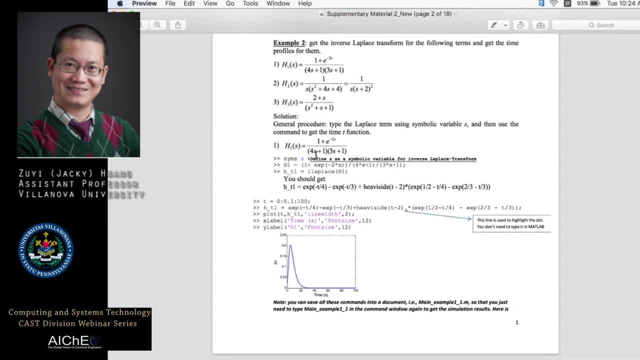 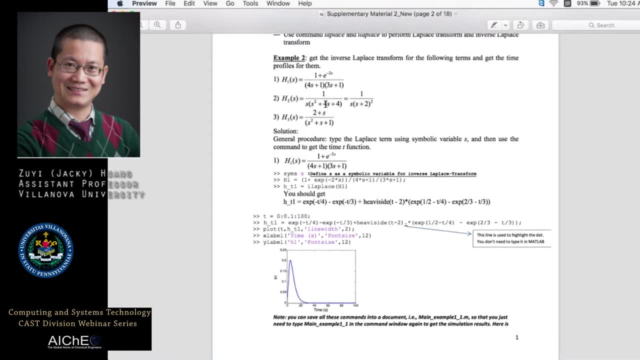 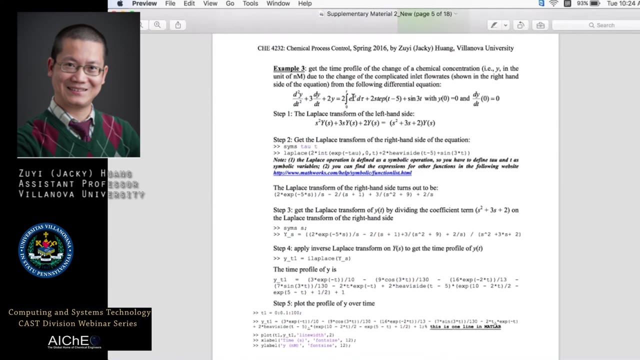 The student there was struggling to solve inverse Laplace transform by hand right And after they learn how to do that using MATLAB, they were very happy And I also showed students how to do the Laplace transform for very complicated right input. 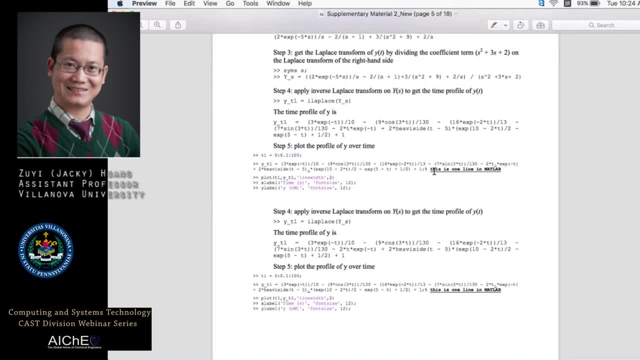 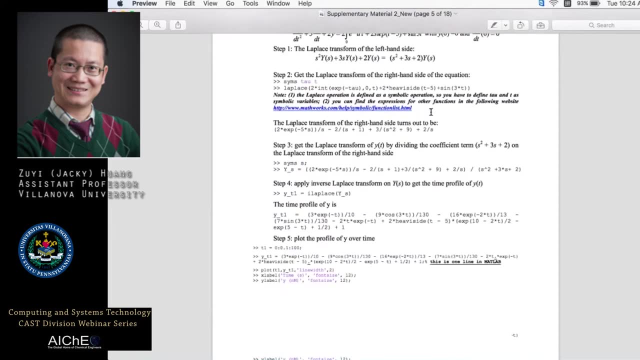 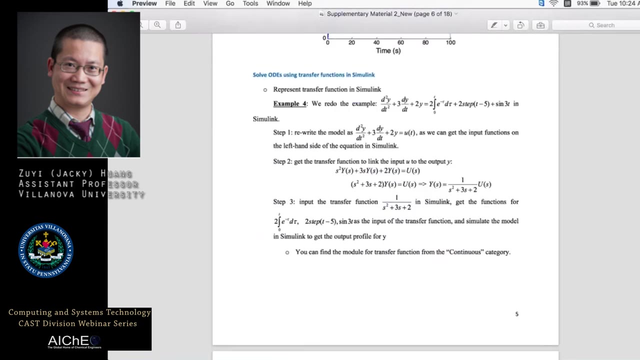 signal and then – so in this approach we just show how to do the Laplace transform. So in this approach, we just type the code in the command window and then I will show the student another approach. Right, I show the student how to – instead of solving the Laplace transform, we represent the model. 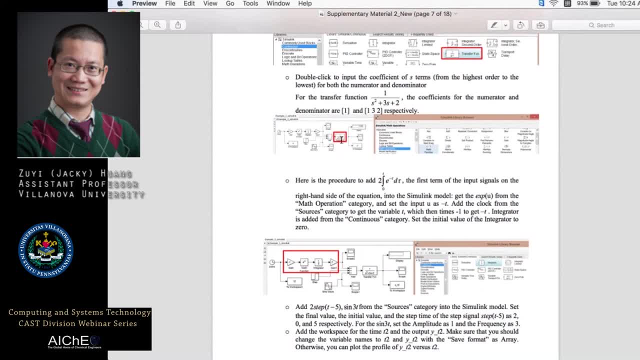 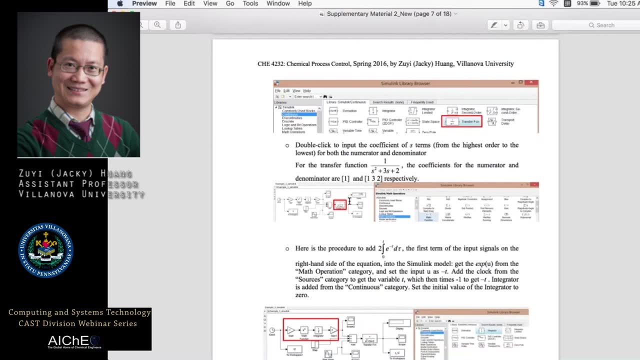 right in terms of function and we represent the signal – input signal- in similar language, so that we don't need to do the Laplace transform of this input signal. So that's another approach. So how to right get out of this? 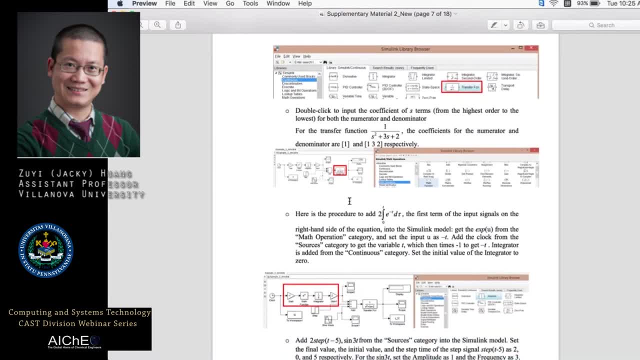 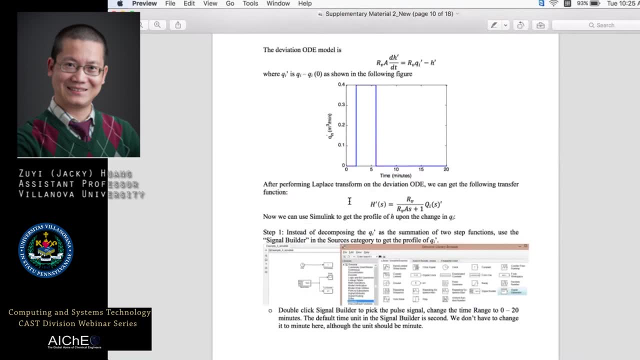 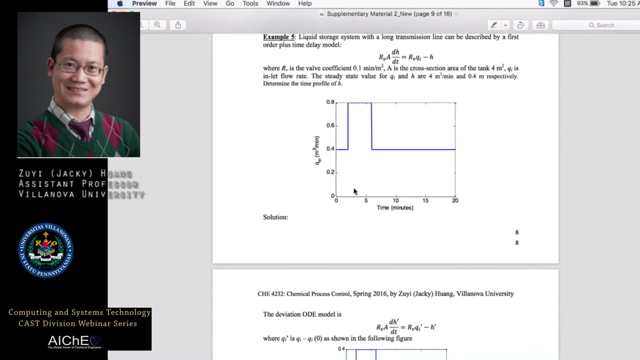 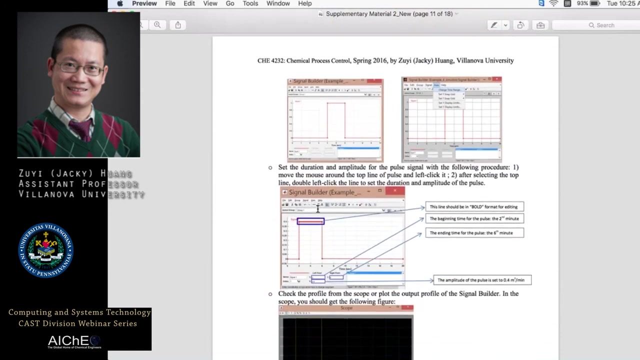 Right: Get the output without solving the inverse Laplace transform in Simulink. So the example – now I want to show you example five and I show students how to – how to create complicated input signal from the signal creator provided by – so actually, 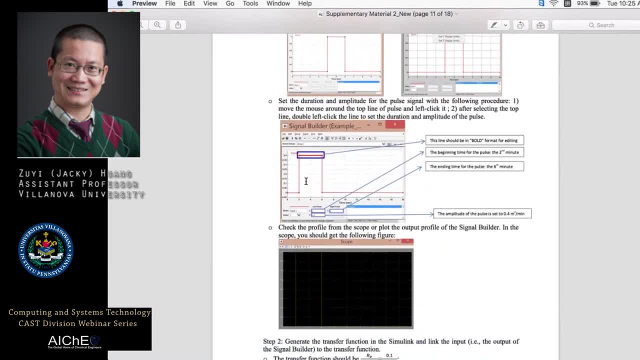 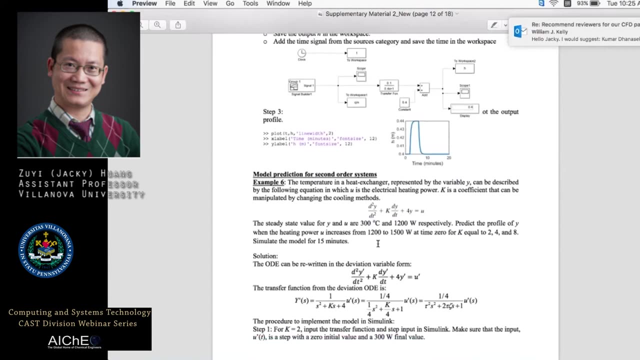 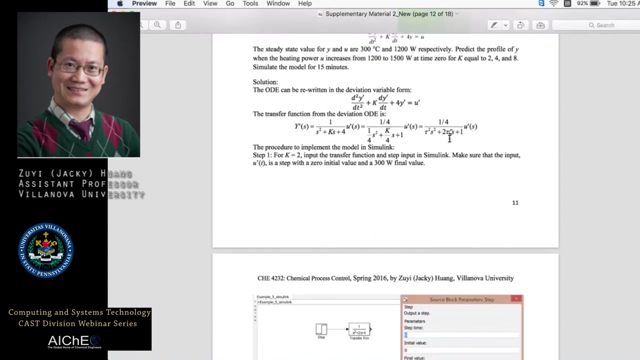 a signal builder from Simulink So the student can build, for example, triangle right and pulse all type of complicated signal here and without solving the Laplace transform Right. And then in example six I show the student right for a second-order system here how 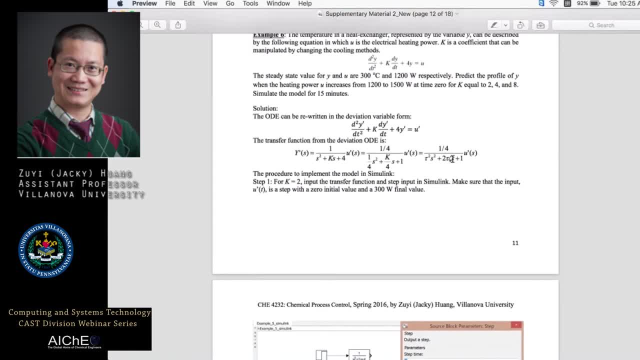 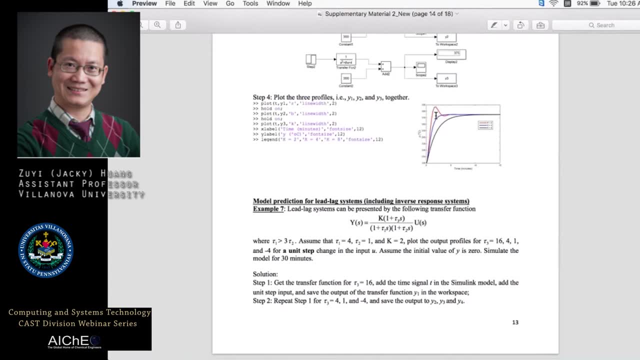 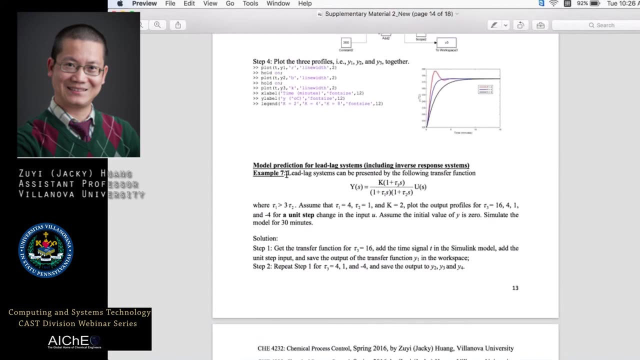 the value of the zeta right. the damping coefficient will change the output, The output profile: right because the second-order system is right. we see the oscillation in the – in the step response And in example seven I show the lead-lead system right, how the time constant in the 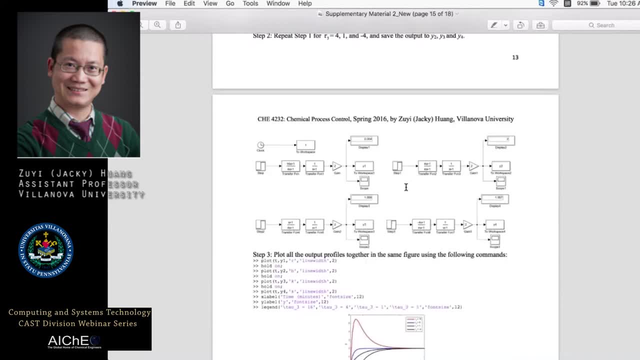 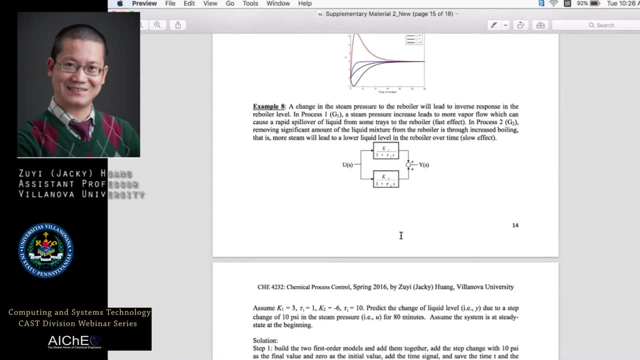 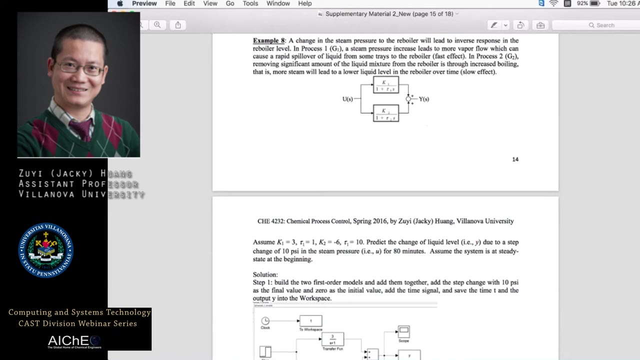 numerator change the output profile. So here we have lead system and we have lead system. And in example eight I show the concept of inverse response Right. So I use the – the summation of two parallel first-order systems to illustrate the inverse. 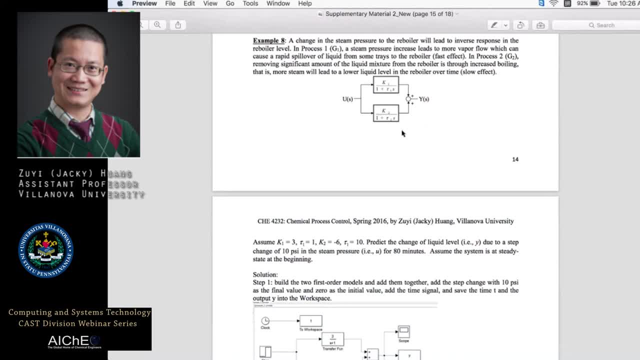 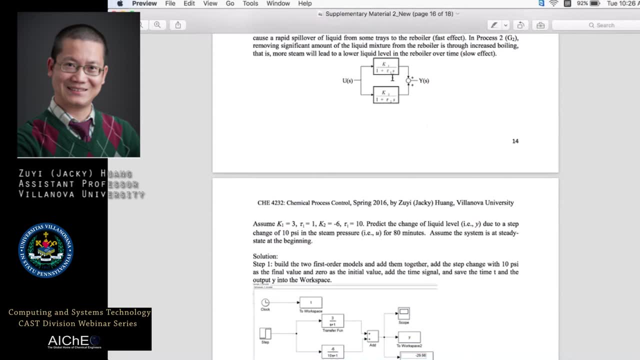 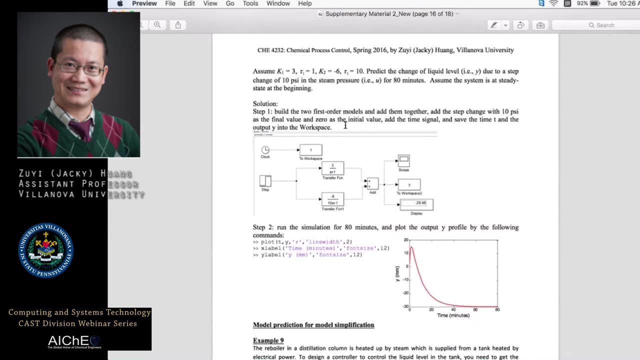 response. So, for example, the K1 and K2, they should have different size, one is positive and another is negative, And tau 1 and tau 2, they should have different – quite different values. So the student, they play around with the K1, K2, and tau 1,, tau 2, and – so that 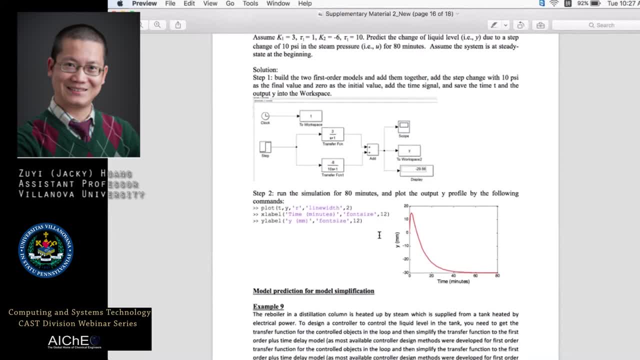 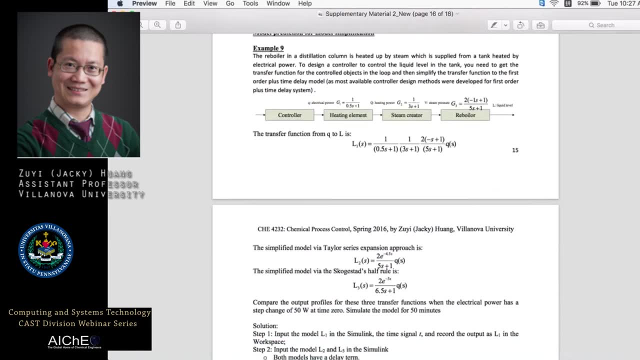 they had a better understanding of the inverse response. And in example nine, and I show the student how to simplify a model: For example the model had more – had higher-order system. For example the model had more – had more than two turns – s-turn in the denominator. 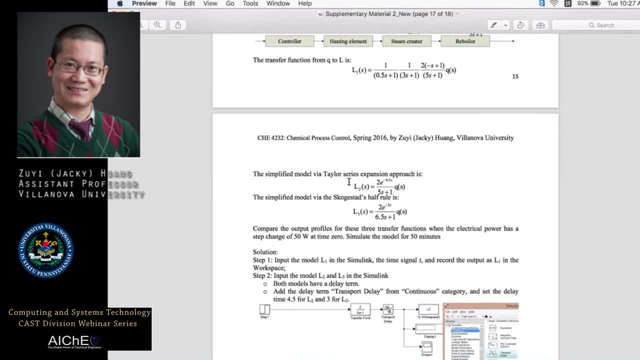 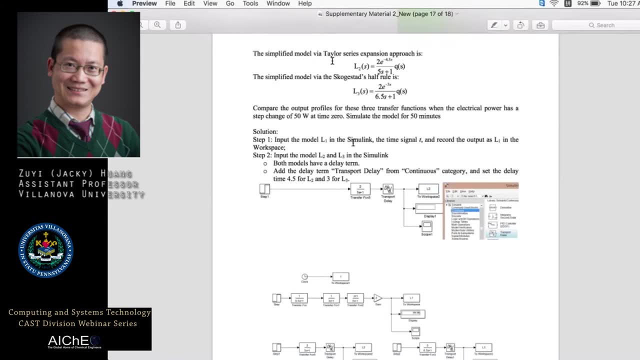 And I show a student how to solve – how to solve this problem, And I show a student how to simplify it, using two different approaches: Right And like – so I'm – as you know, the Taylor series expansion. another one is the 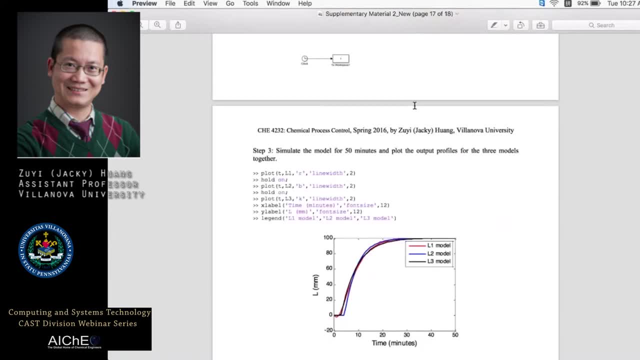 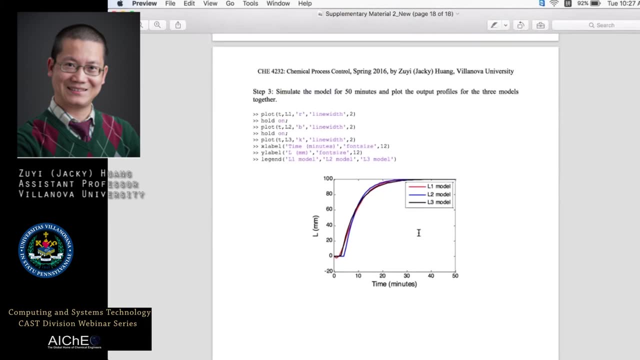 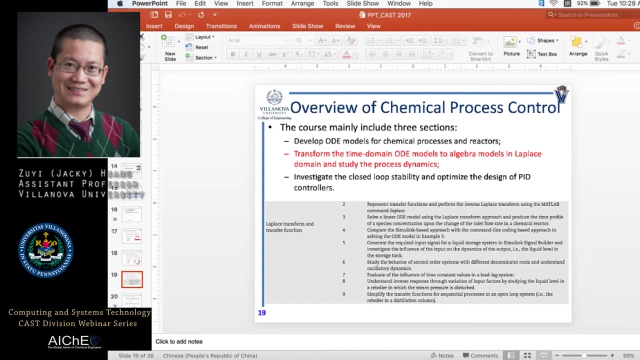 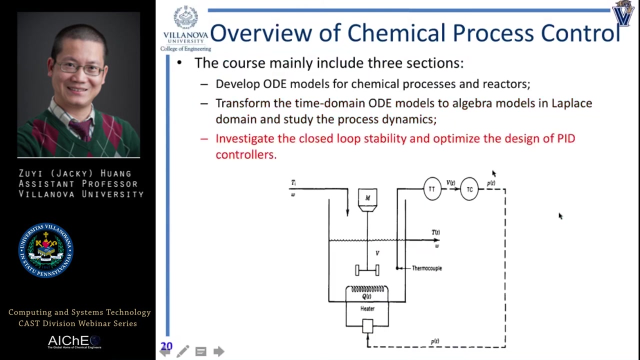 Duster half rule, And then we compare the simulation result from the original model and then also from the simplified model. So, based on that, the student has a better understanding of the simplification. So this is the module two, And then – and then I'll show you the module three. 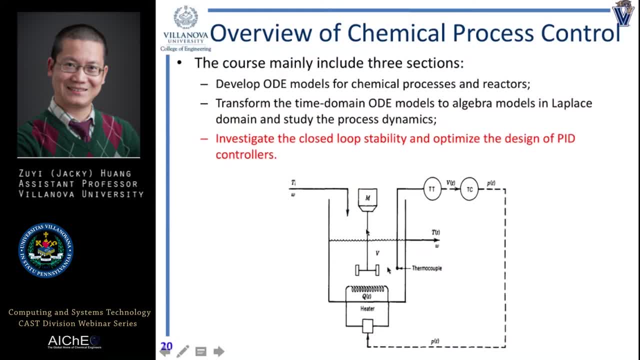 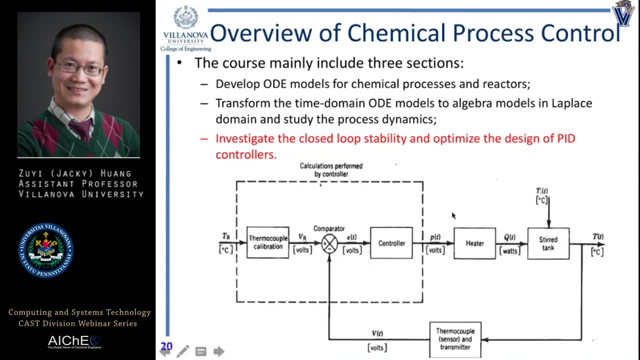 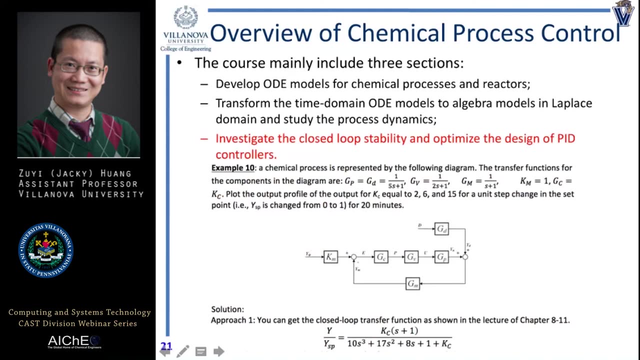 It's more about PID control design. So first I show the student the diagram Right And then how to represent the control system in – in this diagram, And then after that I show – so example ten I show – for example, if I just use 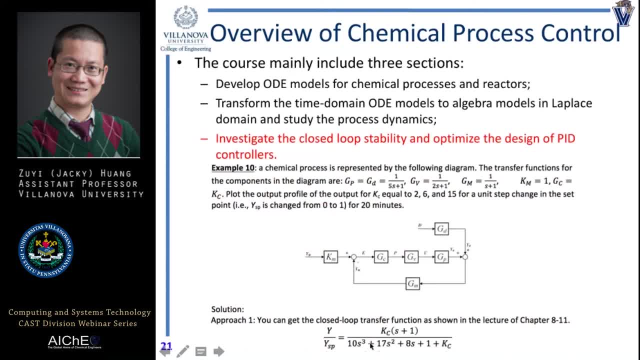 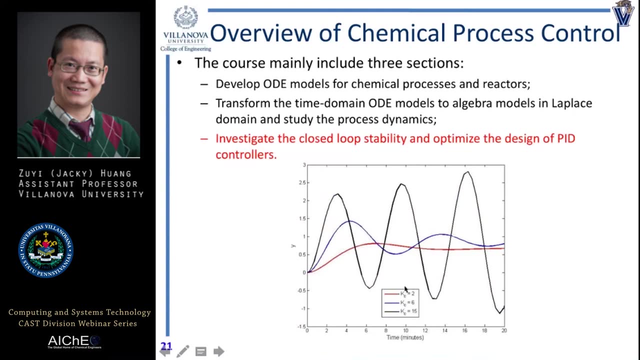 the PID controller Right, And then we get this closed-loop channel function And we could get different output profiles for different Kc values. So we – I want to show the student how the Kc value would change the system's behavior And we could see that if the Kc is too large and the system is not stable. so the student 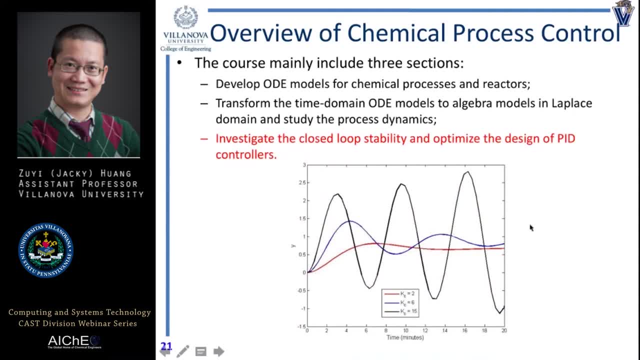 has – has a – have a better understanding of the influence of the – like the Kc – the controller Right On the system behavior. And then I also show the comparison of different PID controller and the P – if you use P and Pi and PID. 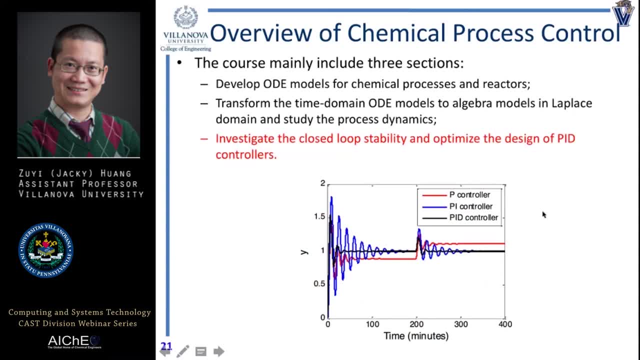 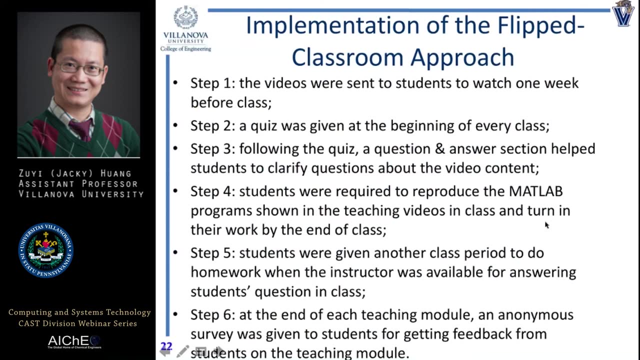 And also I – and student also try different PID tuning method to decide different PID controller. Right, So this is module three. Okay, Now I want to show you how I implemented the flip classroom teaching approach. Okay, So the video was sent to the student one week ahead. 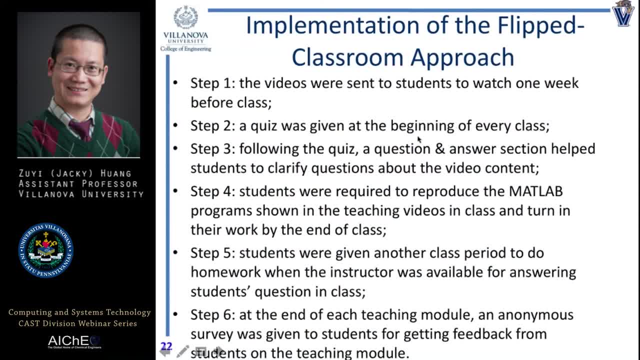 Then, at the beginning of the – the class and the student will do a quiz, But I just want to make sure that the student watch the video The quiz is – is quite simple: If the student watch the video and then they should get a kick, then. 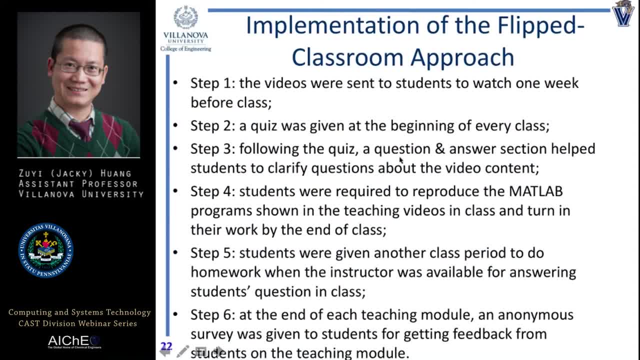 And after that I provide about 10 minutes questionnaire, Question and answer section And if the student have question, So after that the student on the – they will require to reproduce the MATLAB programs in classroom And then after that I provide another lecture. 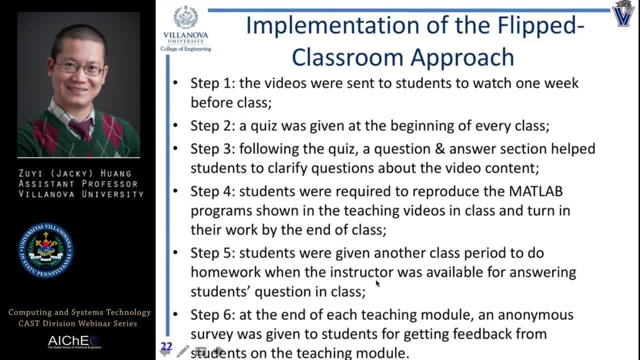 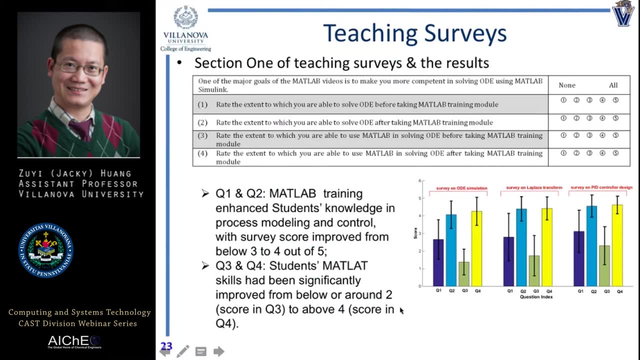 Another – another class time for the student to do the homework, And, after the student finish and the assignment, and then – and they will – they did – they did an anonymous survey, And so now I show you the questionnaires of the survey, also the survey result. 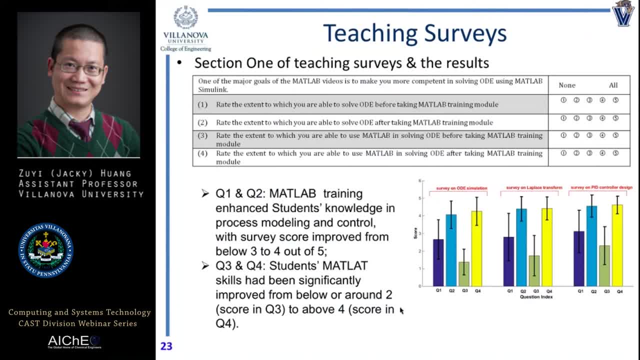 And the survey has three sections. In the first section we try to evaluate student's improvement in the technical skills, And in the second section we want to get some feedback from the student on the inverted classroom teaching approach. And in the last section it's more about open-ended questions. 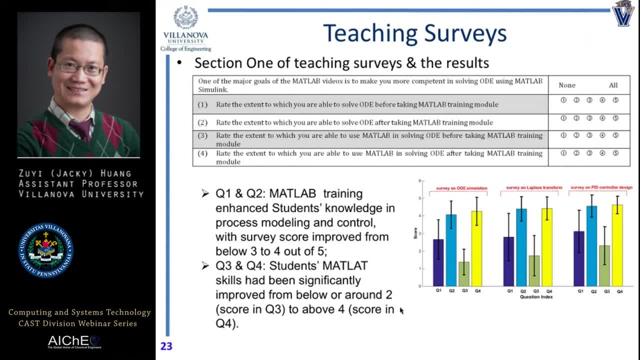 Hey what the student like or dislike: the flipped classroom teaching approach. So now I'll show you the – the – the section one. Write this question here. So we have – so we have four questions: Question one and two: And are used to evaluate student's improvement in solving old problems. 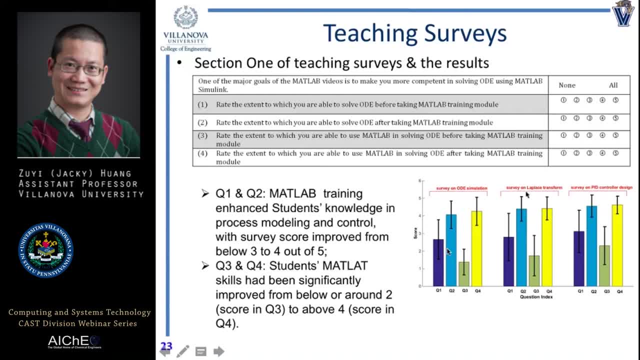 And in – in solving ODE simulation right and in – and doing Laplace transform right and also handling the transfer function And in PID control design. So this one is only for the ODE simulation right, for the PID control design or also. 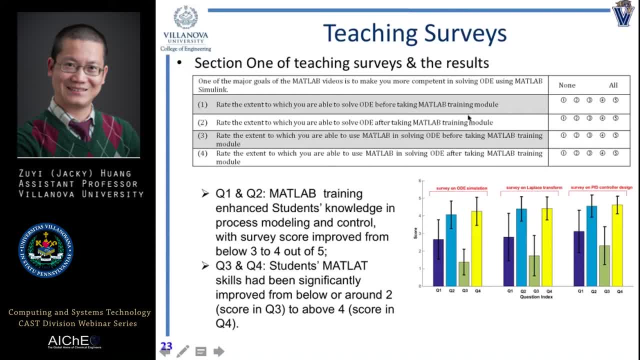 the Laplace transform. We just changed the – right, the technical skills to right accordingly. So we – as we could see well, although the student had learned those technical theory right in classroom and – and that yep did enforce the student to – to learn, 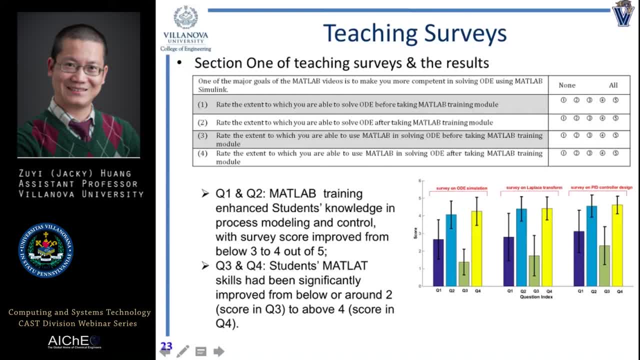 more right and then to – and also to improve their understanding of those theory. So in problems three and four, And we want to evaluate student's improvement, We want to evaluate student's math – math skill to solve ODE right and also Laplace. 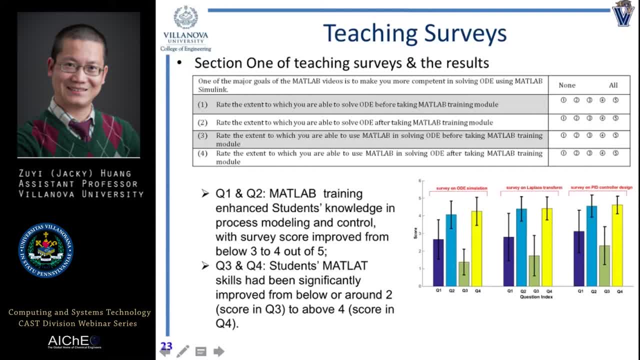 transform, and then the PID control design And so again, right as I mentioned before, right student they – they did not learn math yet that much before they take – they took my course, So therefore you could see – so before they took the – the three teaching modules. 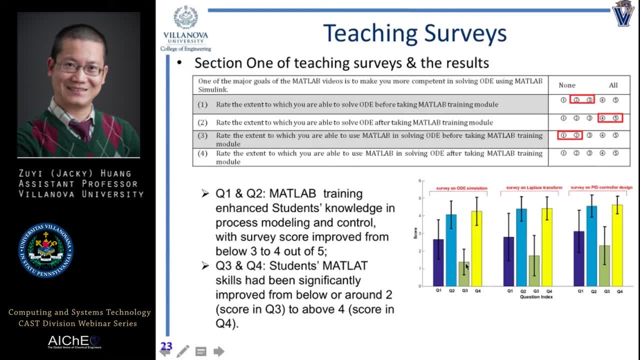 right the – the MATLAB skill is low. Actually, you could see the MATLAB skills increasing in question three right from module one to two and three, because they learn more and more MATLAB right And then, yeah, so after they learn – after they took the – the teaching module right. 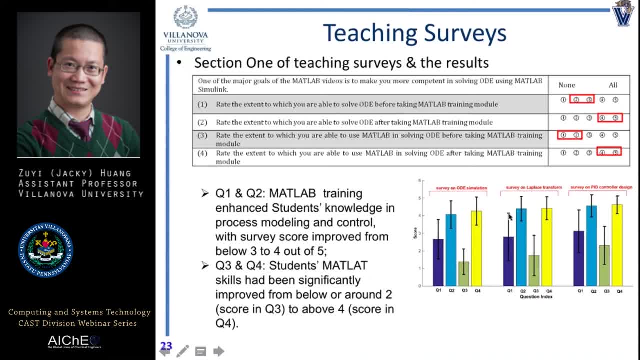 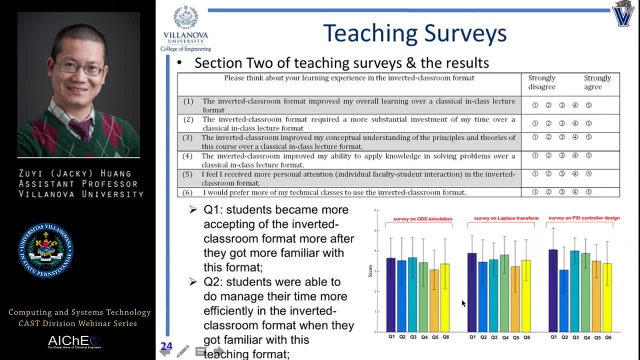 and – and did the MATLAB assignment and they – they are quite kind of confident with the MATLAB skills. yeah, So this is session one about teaching modules. Thank you, And now for the master teaching survey. now let's talk about student's evaluation. 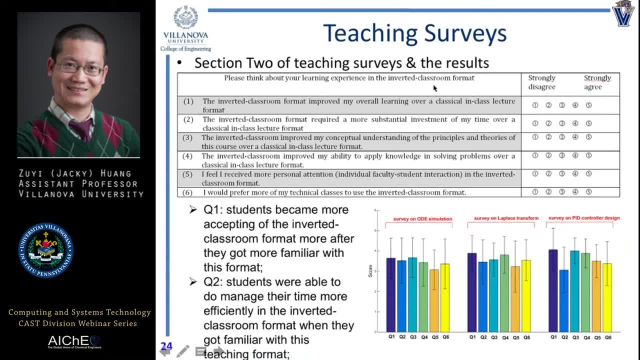 of the flipped classroom teaching approach. So one meets this totally disagree – agree. and five meets strongly disagree – strongly agree. All right, The first question is: the inverted classroom format improves students overall learning and you can see from all three teaching modules and that score is – the students score is. 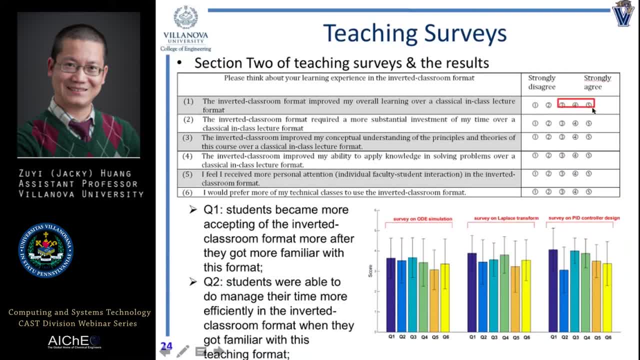 The students score from 3 to 5, and it's quite positive. So the second one is the free classroom format- require more time to do the work. Actually, the students, they did think that they spend more time in the free classroom teaching format. 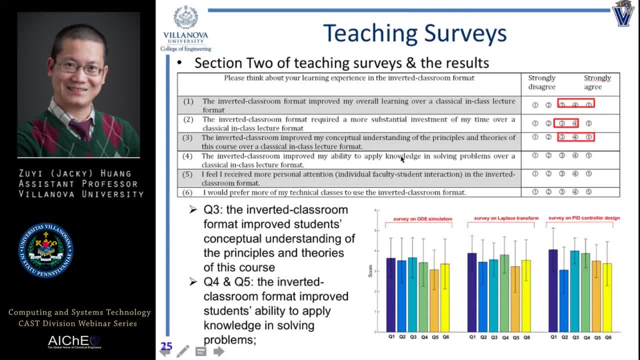 And number three is the free classroom approach improves the student's understanding of the principle and theory. So again, you can see from this question three for all three modules and the students. they did think that the MATLAB experience can help them to understand more the concept. 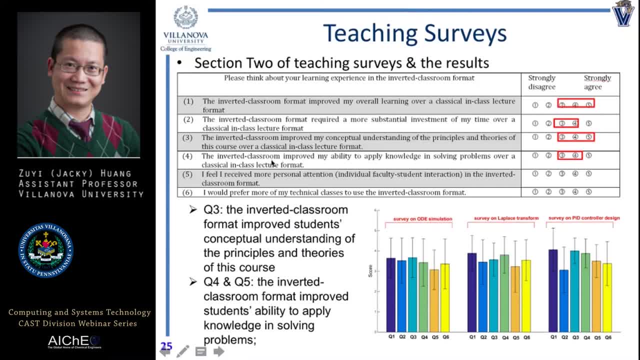 Question four is the free classroom approach improves students' ability to solve problems. So you can see after question four here and the students become more confident to solve problems. And so I talked with some students. They told me that they feel confident because some of them. 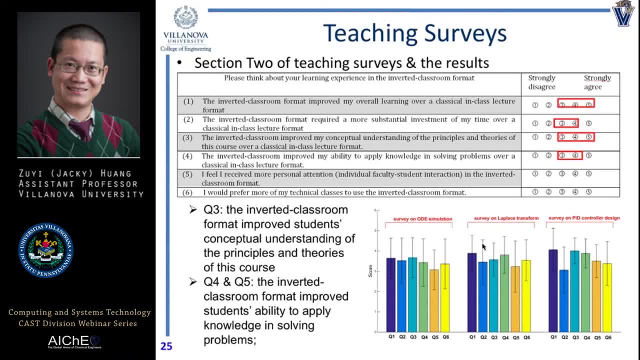 actually they didn't know. They didn't know how to solve the problem by hand, but they do know how to solve the problem by MATLAB And so they like MATLAB after they finish all the training. At the beginning they quite resisted the MATLAB. 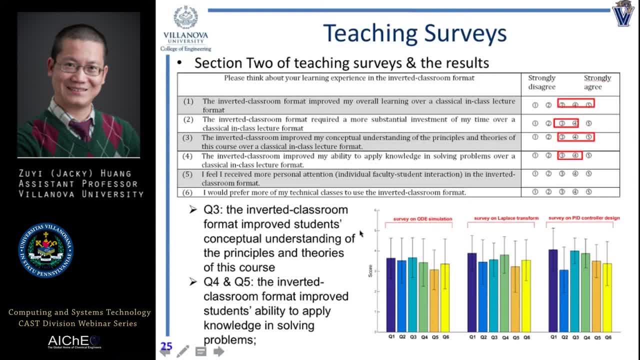 because they learned little MATLAB before they took my course And problem five and the student received more personal attention in the free classroom approach. The score also is positive. And last one is The student recommend more recommend the free classroom approach to other courses. 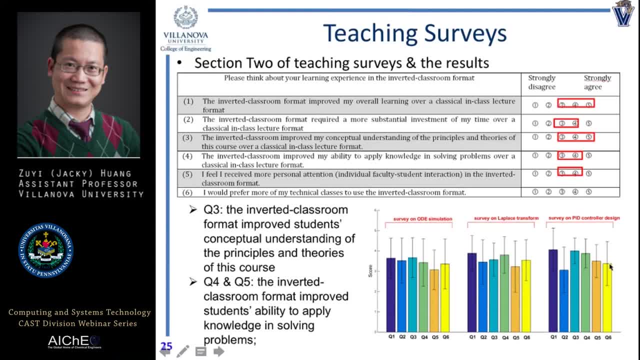 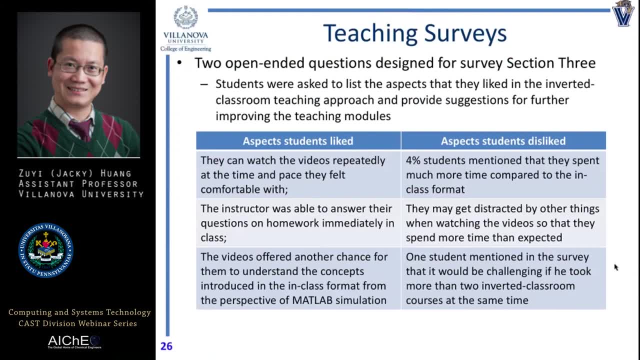 So actually they recommend this teaching approach to other courses. Well, here's question three. It's an open-ended question Again. well, we can make everyone happy, right? Some students- they like it- like this teaching approach, but some they don't. 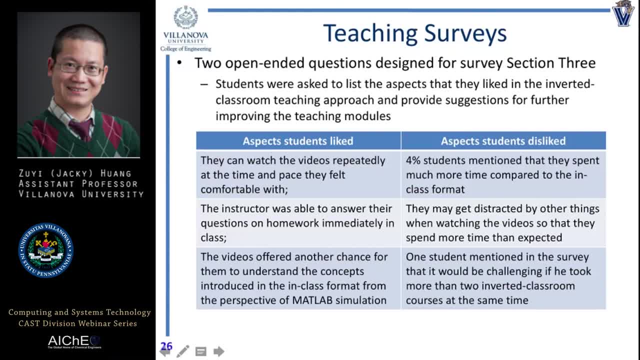 So here's some examples. They like the free classroom approach because they could watch the video anytime, anywhere. Also, they could ask the instructor questions when they do the homework. Also, the MATLAB module help them to learn the materials Well- the aspect of the student they don't like. 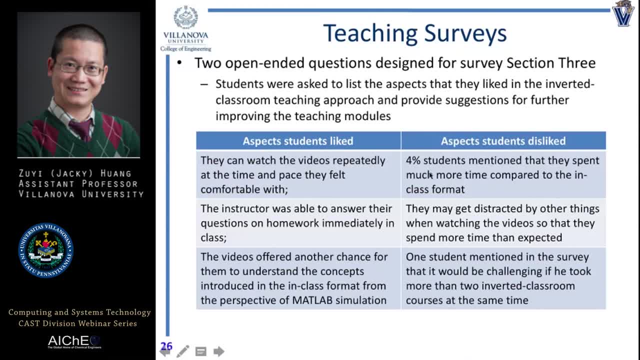 and the free classroom teaching approach is several students. but the student mentioned that they spend much more time in the free classroom teaching approach because they have to watch the video, like they have to watch the video before the class and at the same time they also have to attend the class. 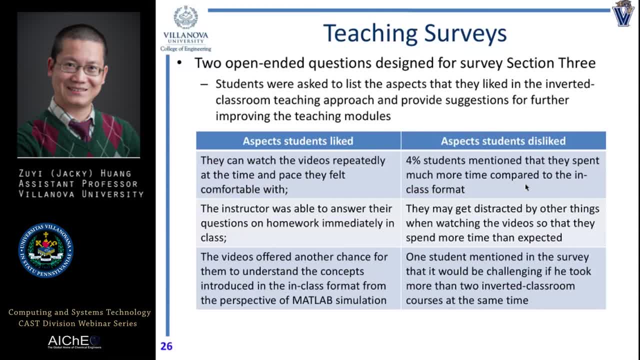 So it seems that they have more time to stay with the instructor And also the student. actually, one student mentioned that it's very challenging for him to take more than two free classrooms. So it's very challenging for him to take more than two free. 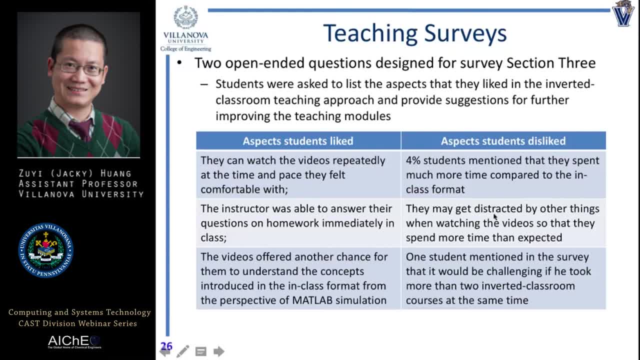 classroom courses at the same time. Also, some students complained that they got attracted by other things when they watch their videos, like because the instructor is not staying with the student. they could do whatever they want. Anyway, this summary of the project tool. 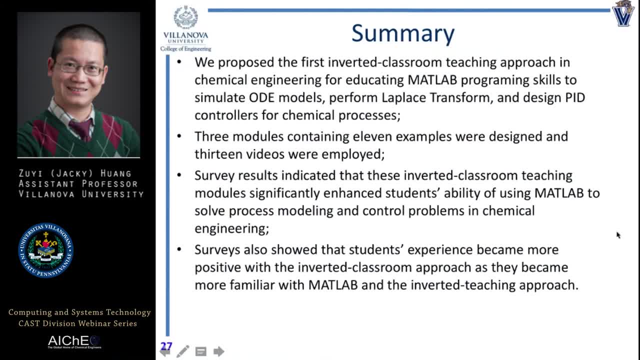 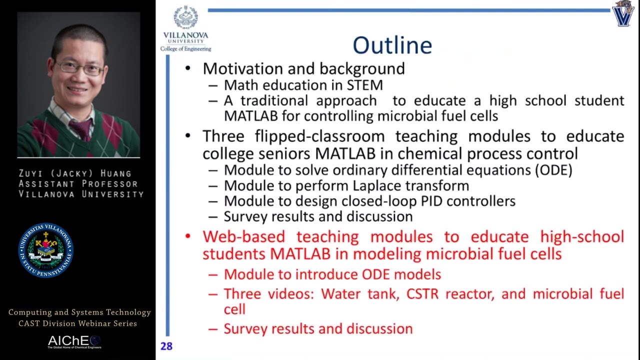 so we developed a free classroom teaching approach and the survey shows that the student they were quite positive with the free classroom approach And also the student's skills of using MATLAB have been significantly improved Now. so I shortly introduced the last project. 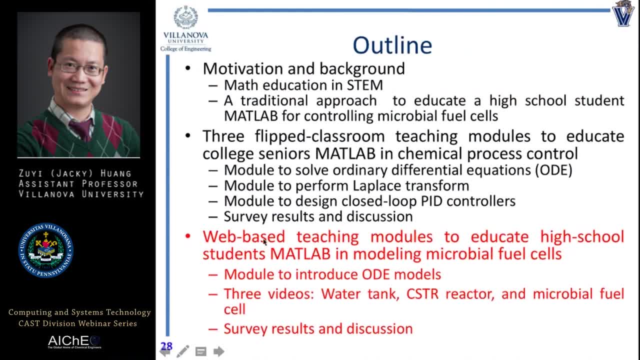 I hope it's about web-based teaching approach to educate high school students in MATLAB in modeling macrobial field cells. As I mentioned before, this is an extension to the project one and we just We changed everything to the web-based format. 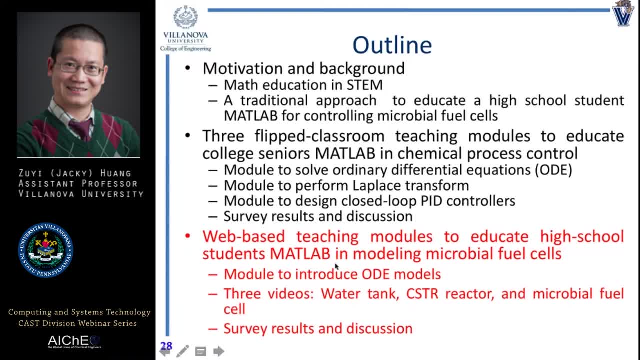 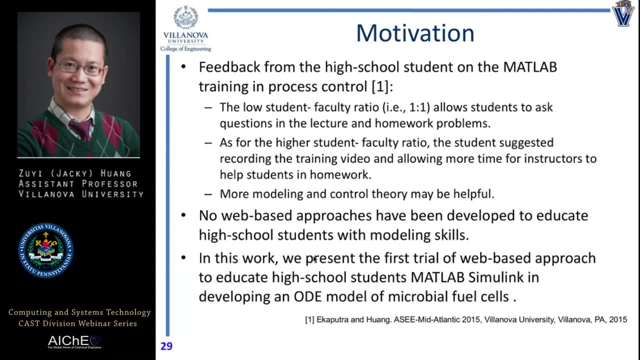 Actually, the web-based format is not pure free classroom teaching format, but they are similar. So I say it's still. We got this as a free classroom approach. So here again, this is motivation and I want to get more students attracted by this project. 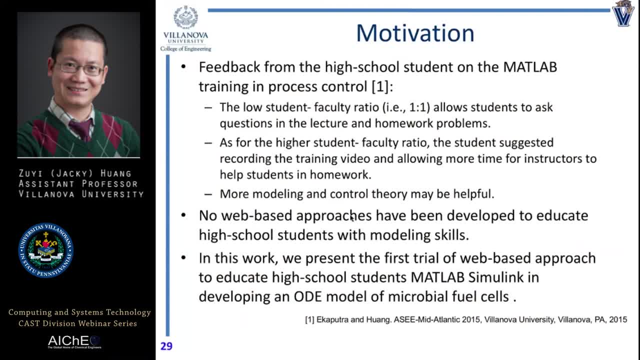 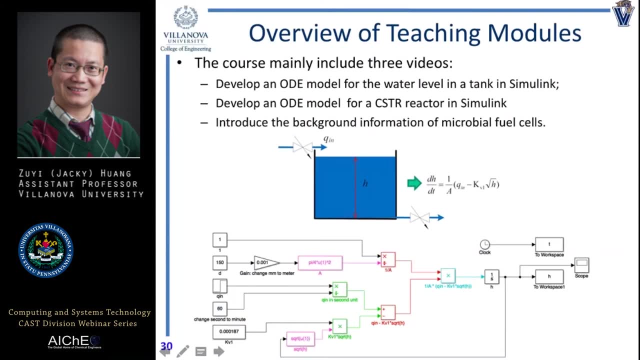 and to to all students at the same time and also provide facilities to the students, but that's why I recorded the teaching modules. So here I only have three videos in this project, And the first one is I showed ODE right. 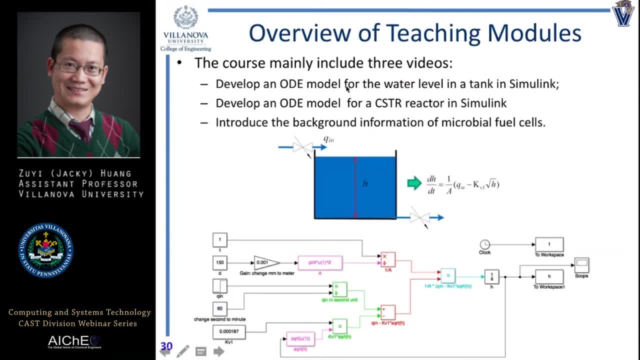 because some students they don't know what ODE is. And then I showed students how to develop the ODE model in Simulink for this program. Yeah, I see In this water tank example- this is a very simple example and then the students feel: 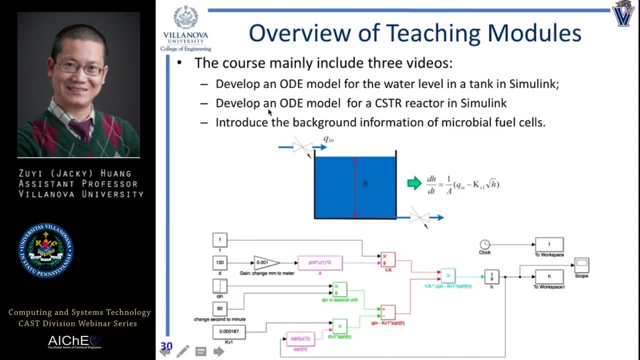 more confident, And after that I showed the students step-by-step how to develop the OD model for the CSTR model I showed you before That's a more complicated one After the students finish this complicated CSTR model, and then I introduced the background. 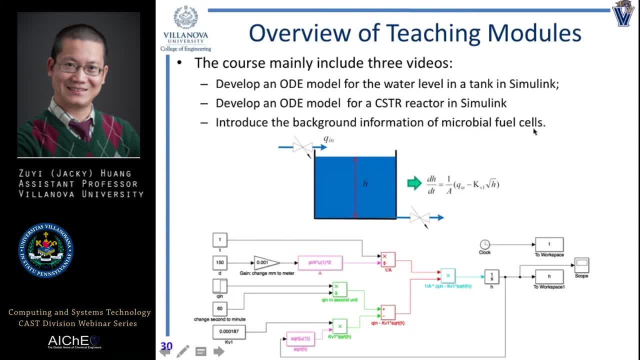 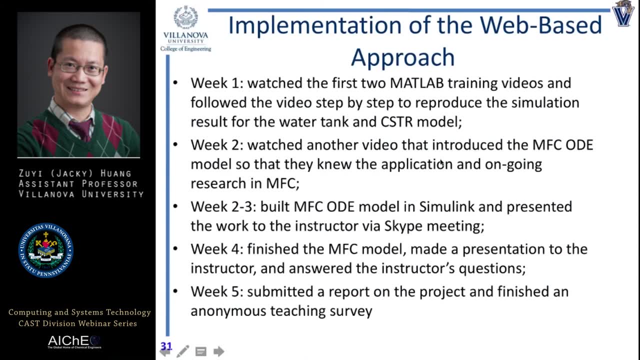 of microfusil, also the OD model of the microfusil, and then the students began to do the project. This is how I implemented the web-based teaching approach, and actually the students only worked for four weeks on this project. 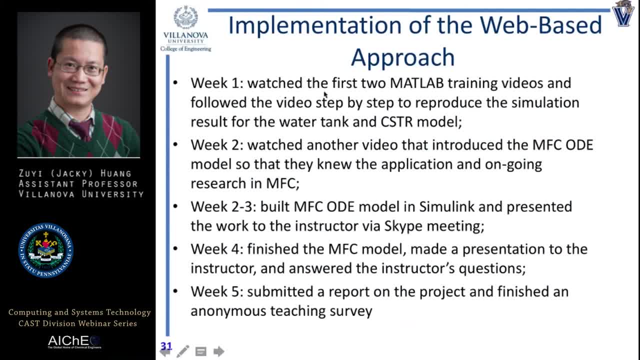 In the first week the students watched the first two maillette training videos, and one for the water tank and another for the CSTR. It's a bit difficult for the CSTR model and then the student reproduces these two examples. 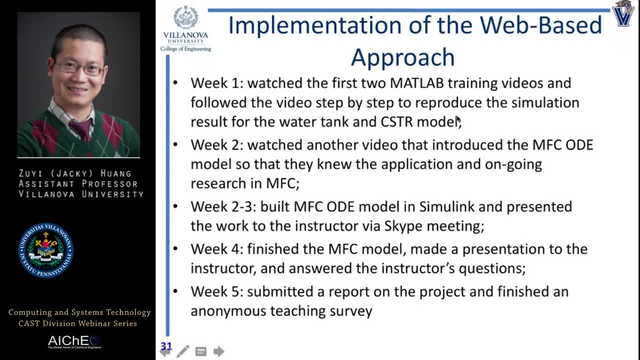 just step by step and then send me the results on Friday, And then I organize a Skype meeting with each student and then in week two the student is going to watch the introduction of micro-B2CELL ODE model, and after that the student just works on the micro-B2CELL ODE model project. 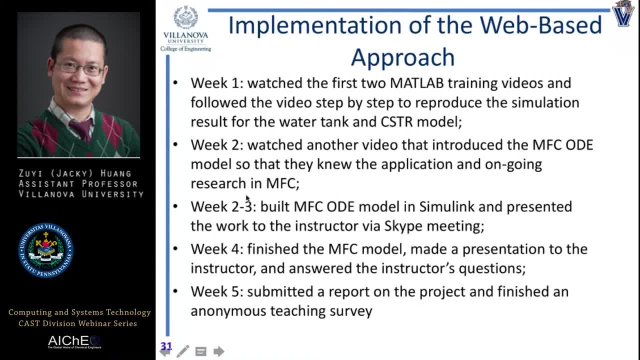 And on each Friday from week two to four, I organize a Skype meeting with the student. I also use the TeamWeaver. In the TeamWeaver I could help the student to debug the CSTR model. I also use the TeamWeaver. In the TeamWeaver I could help the student to debug the CSTR model. In the TeamWeaver I could help the student to debug the CSTR model. I also use the TeamWeaver. In the TeamWeaver I could help the student to debug the CSTR model. I also use the TeamWeaver. In the TeamWeaver I could help the student. 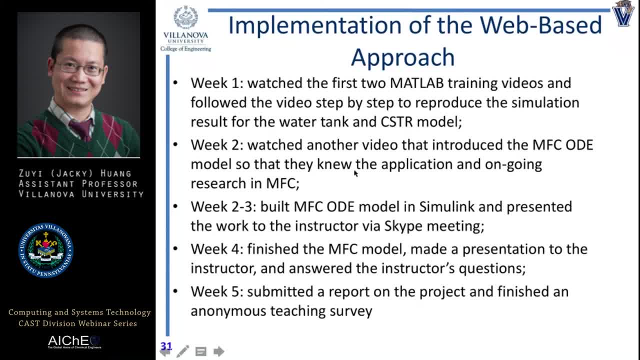 to debug the CSTR model. I also use the TeamWeaver. In the TeamWeaver I could help the student to debug the CSTR model and then in Most student and they were able to finish the project at the end. 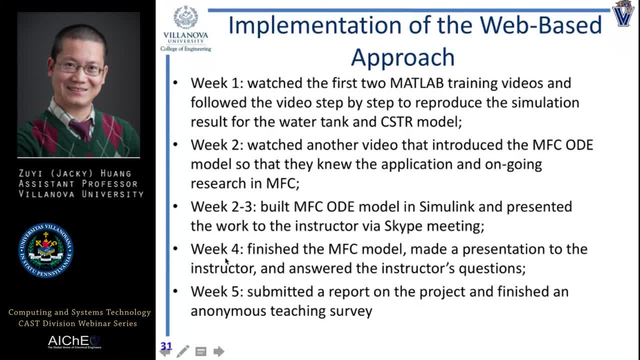 of week 4, and then weeks 5, and they're going to submit a assistant report, and I also asked them to do anonymous teaching survey. Well, you might ask me how much time they spend in each week. Actually, I 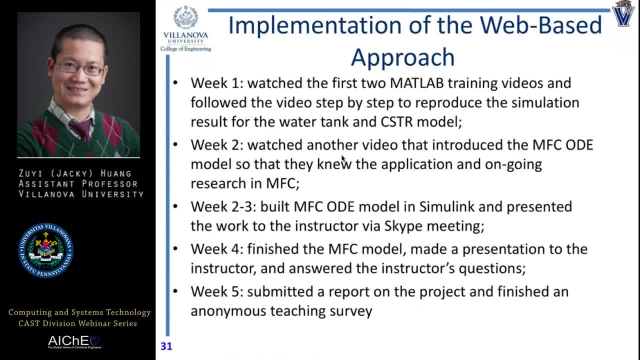 I did not check their time but I did do the survey and how much time they spend in each week. Typically they spend four to eight hours per week and it depends on the student's ability And for the teaching survey I tried to make it anonymous. 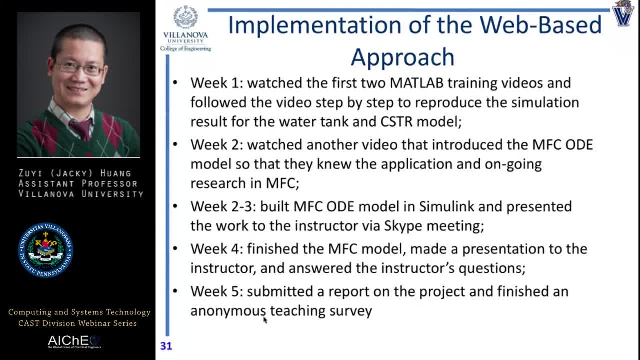 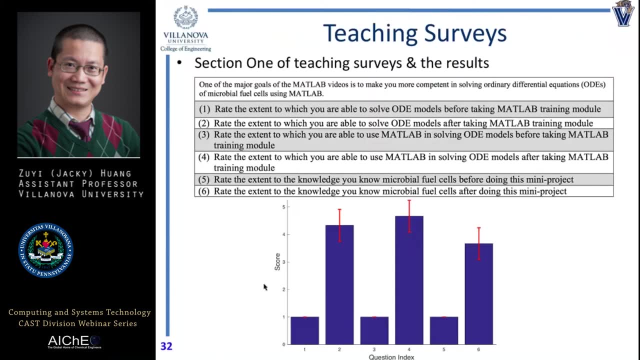 So what I did is I asked the students to send their surveys to my wife's email, and then my wife printed the survey and then handed the survey to me, so that I didn't know who did the survey. Okay, so here again. similarly, we organized the survey in this section. 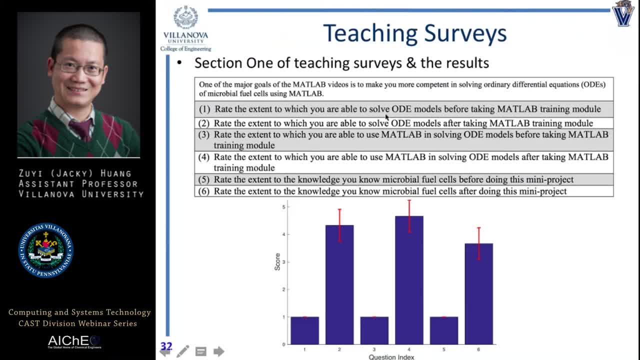 In the first section it's more about the technical right, for example, how the students' MATLAB skills improved. so one and two- again all students. they did not learn MATLAB before the survey. They took the project and joined the project. so you can see the MATLAB skills have improved. 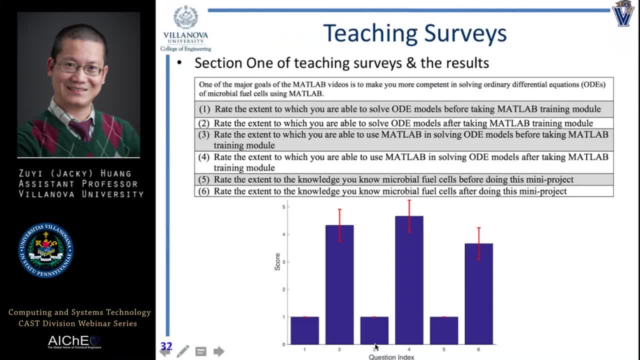 And then also actually three to four is MATLAB skill, and one and two is their ability to solve ODE. So the high school students: they don't know how to solve ODE before they did the project and after that they know how to solve ODE. so one and two is about ODE solving, and three 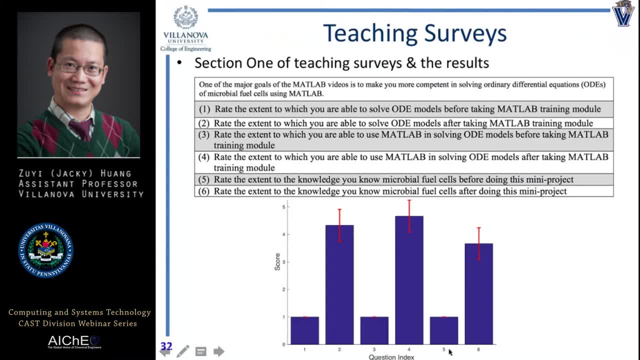 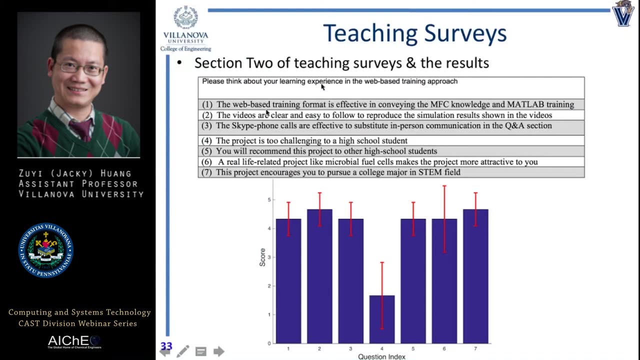 and four is MATLAB skill, and then five and six is their knowledge of micro-bit fuel cell, And you can see that after they did the project, their skills have been improved. And then section two is more about the web-based teaching approach, and the first one is the 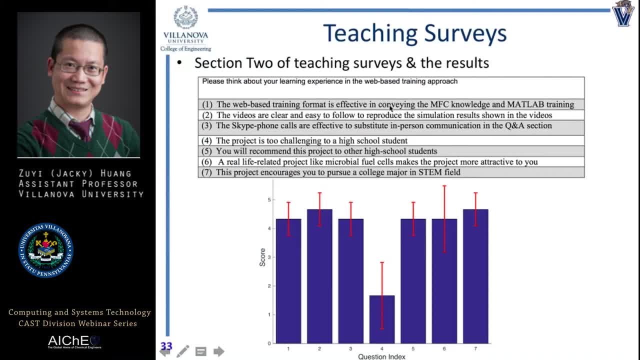 video, the web-based approach, and effectively. The second one is the video and it's all clear and easy to follow. and number three is the Skype meeting and you can help students to answer the questions. Number four is the project is too challenging to a high school student, so most students. 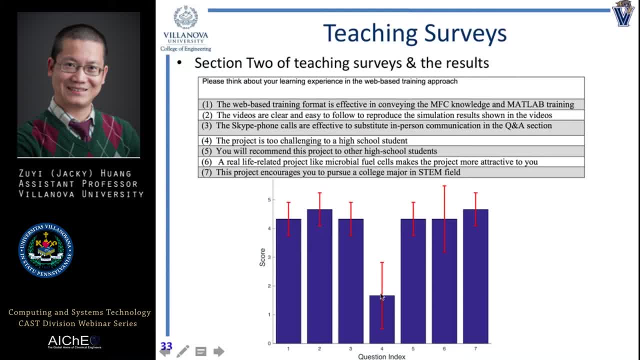 they say they're a problem and the project is not that much challenging. This is out of my expectation. Actually, the project should be challenging, But anyway. and number five is the student will recommend this project to their classmates. Number six is the micro-bit fuel cell project. and very interesting and help them to stay. 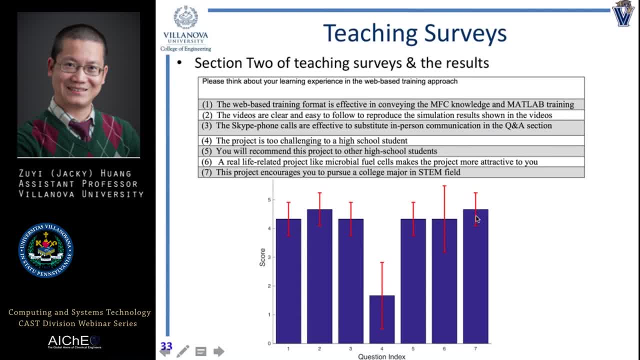 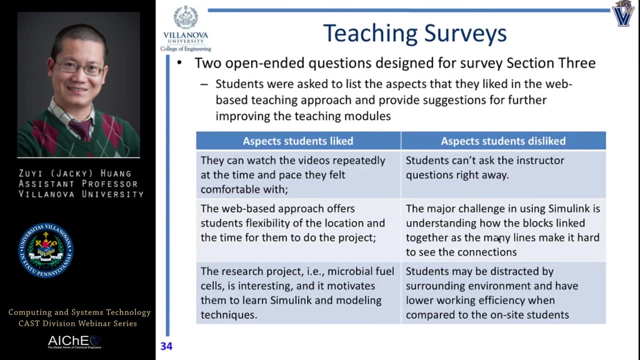 in this project. And number seven is the student will this project helps them to stay in the STEM field. Actually, all the students, they pick the project. And number eight is the student will pick the STEM field major after they finish the project. 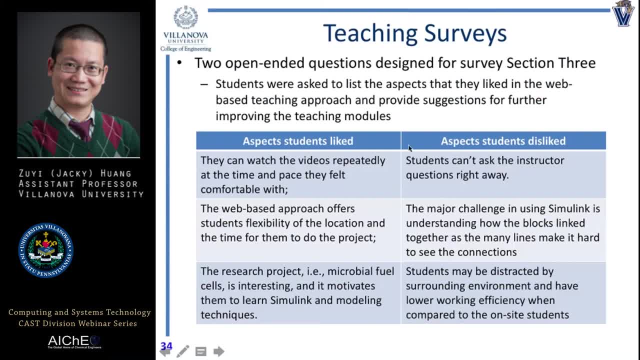 So here is just a brief overview – instruction of the question three, right of the set of questions three, what they like and don't like and the web-based approach. Similarly, they like the web-based approach because it provides the flexibility to the. 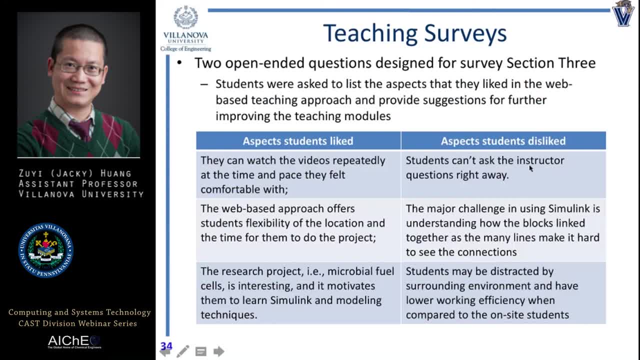 student. What they don't like is they can't ask the question right away. They can't answer the question immediately. So when I teach a test, my students always do not ask the question right away. And then the symboling, especially sometimes if the model is complicated, there's so many. 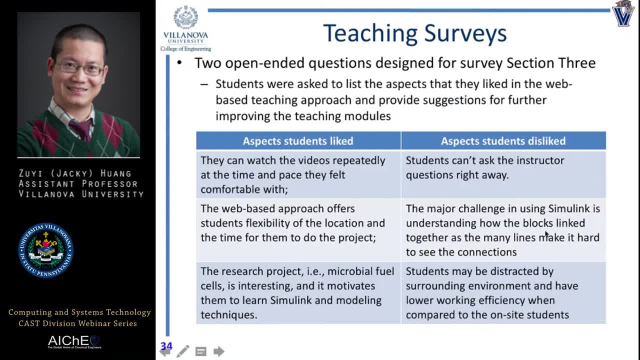 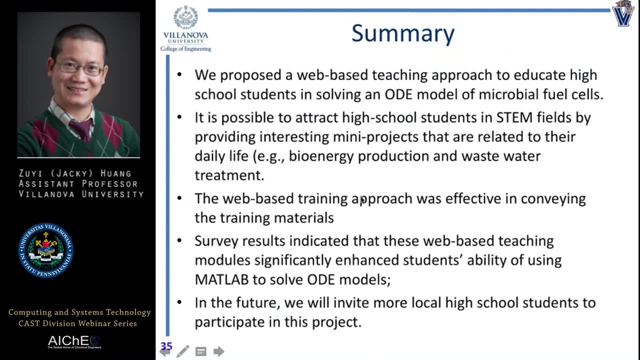 lines in the symboling. it's very difficult for the student to find what's wrong in their model. Here are some of it. So we developed a web-based teaching approach to educate high school students and then all students finished the project and they did a good job and they got offers from top. 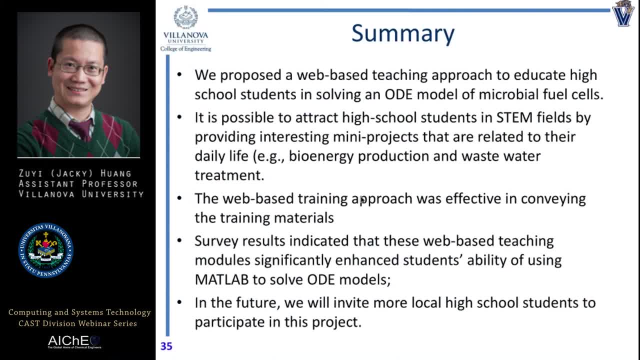 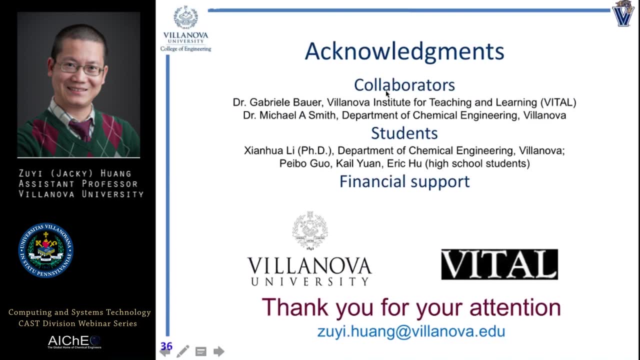 school, like Cornell, UCLA and University of Michigan, and all of them stayed in their major. So in the future we will invite more local high school students to participate in this project. So here I appreciate the help from my collaborators at Renova and also my students, great students. 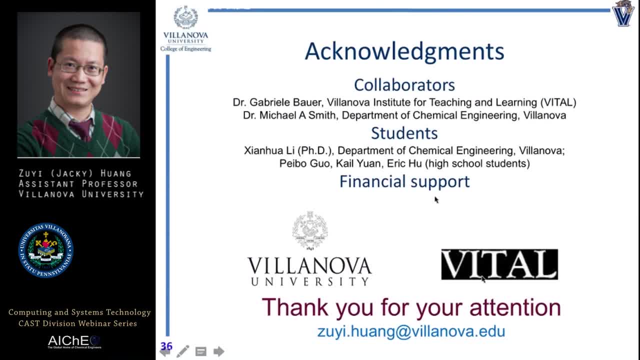 and I also appreciate the financial support from Renova And especially thank you, Especially the VITAL, the VITAL, the Renova Institute for Teaching and Learning. Thank you for your attention. Any questions are welcome and, again, if you can ask me questions on the webinar, you can. 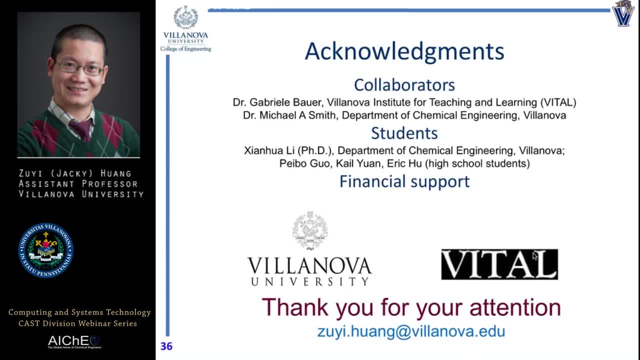 send me email or you can also visit my website and all the handouts and videos are there. Thank you, Fantastic. Well, thank you for that presentation, Jackie. Excellent. not only experience, but you showed quantified, quantifiable results on how they've you know their reaction to the class. I just 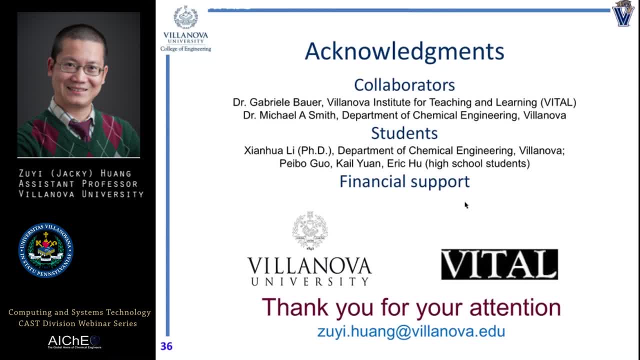 had one one question on. you mentioned something very interesting, which which was that, in general, students are looking to try to get more information more quickly. you mentioned that some of the students said it took longer for them with some of the flipped classroom approaches. do you think that's a problem? 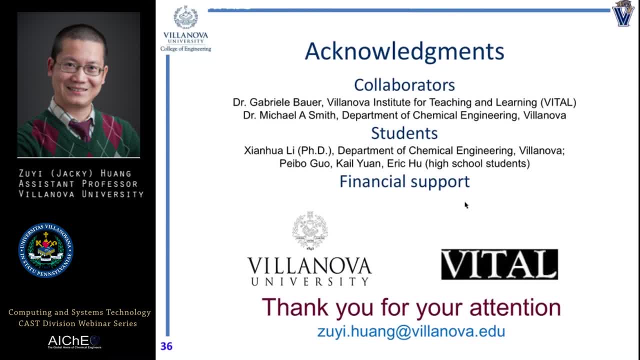 do you think it? I mean, they obviously are learning a lot more that way. what are some ways that we can potentially make it more time-efficient with the flipped classroom? well, very good question. um, so the students they come, they saw they spend more time because they have to spend the same right they? 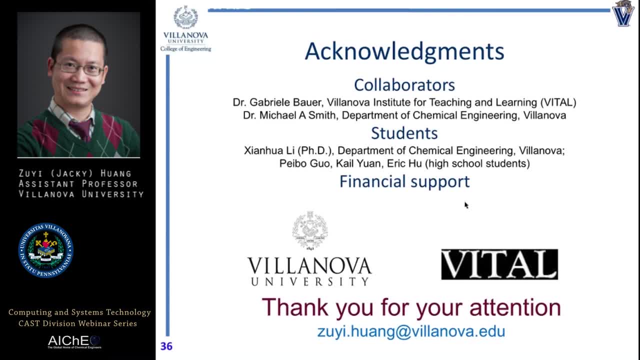 had to spend the same time with the, with the instructor, but someone had to come to classroom to do the homework and also to have to watch the video. um, and that that's why they think and they spend more time and element is they, they got distracted cause somebody watched. 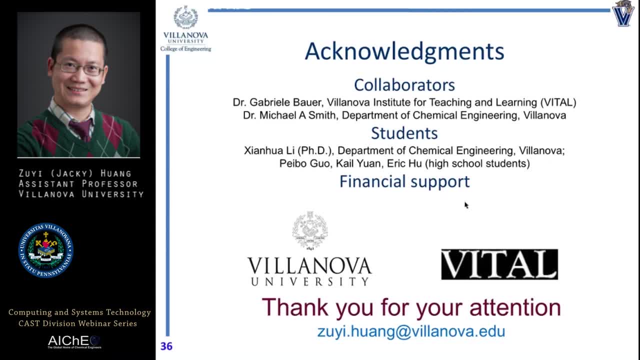 the video. um, right in the morning, and then they do. they don't make just not gold. and hey, get up and make and write video. that's what together, much, together, right. and then a student day, and then they watch the video. I light up fancy fesney. 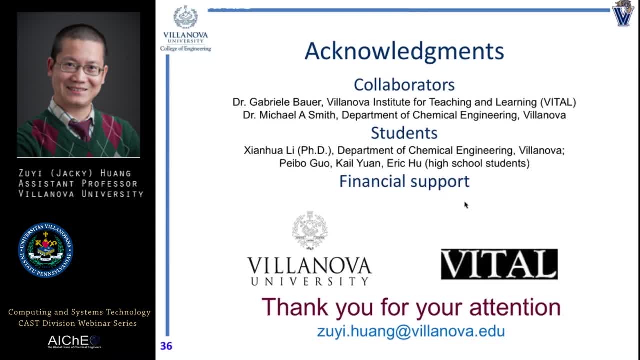 and then come back and then they had to watch the video again because sometimes he just forgot. So some students were complaining about this and they got distracted. So one way to improve the efficiency: maybe we could put peer students in groups and 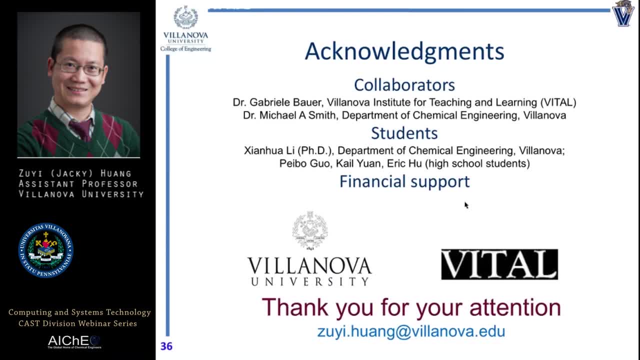 then they watch the videos together. For example, five to six students as a group. they had to fireplace and then watch the video together so that they don't get that much distracted. I think the distraction is the issue And, to be honest, well, I talked with some students. they do these things- that the total